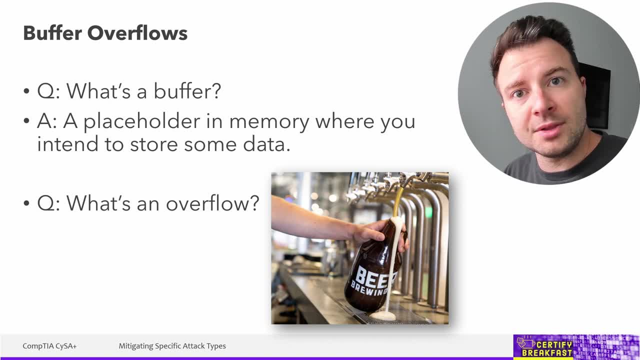 It depends on a number of factors and it depends on whether the overflow was accidental or was intentional. So in order to understand what all the possible effects, the possible outcomes of a buffer overflow can be, we need to take one step back and look at the big picture here. 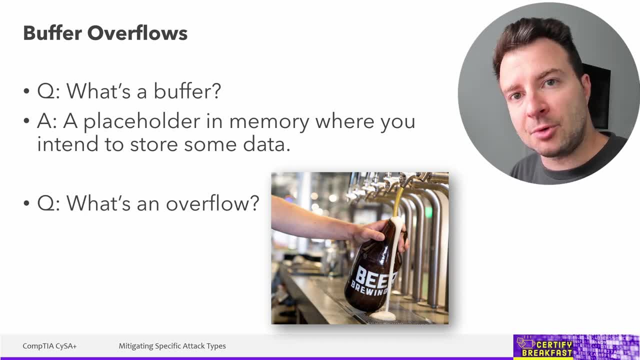 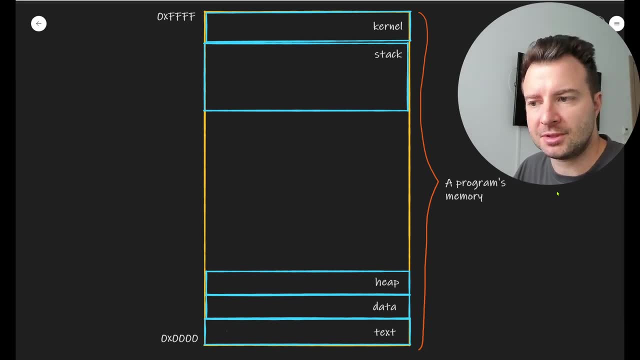 Start by looking at how a program sees its memory when it first starts up. All right. so this right here is just a slightly simplified representation of how a program sees its memory as it is allocated by the operating system right after that program starts, And the memory is a linear space which 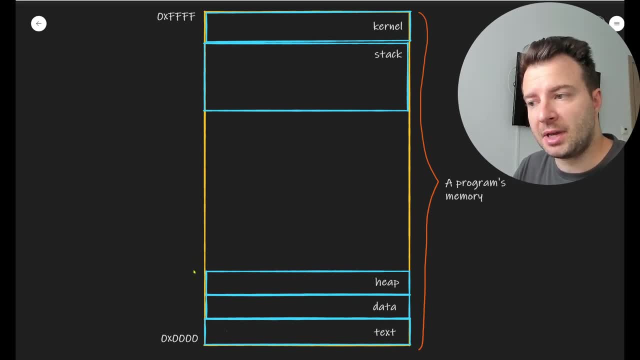 means that every position in this memory space has a specific address, And in our example here we start from a theoretical zero address here at the bottom up to a maximum theoretical value right here at the top. Now, the real values, of course, are much higher than this because we need to address a large amount. 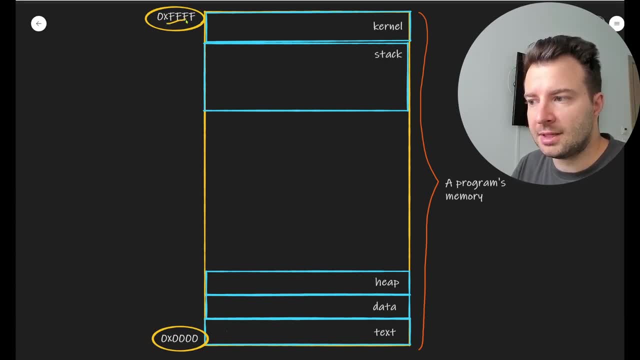 of memory nowadays, But generally we will be using hexadecimal digits, just the one that you see here, to represent memory addresses, for two reasons: First of all, because they allow us to write addresses using less characters, and also because the hexadecimal system allows us to use 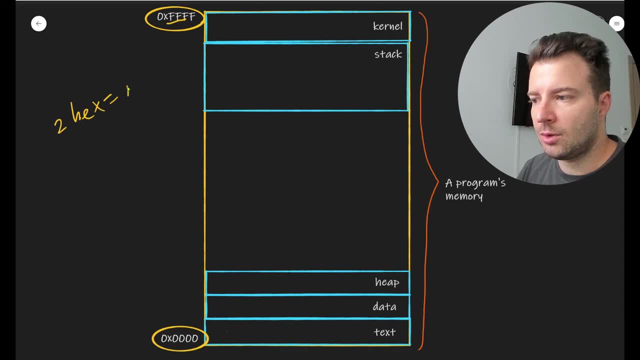 two hex digits to represent one byte, And that's actually because each hexadecimal digits ranges from zero to nine, followed by A through F. So with two digits we're going to end up with 16 times 16, which is 256. 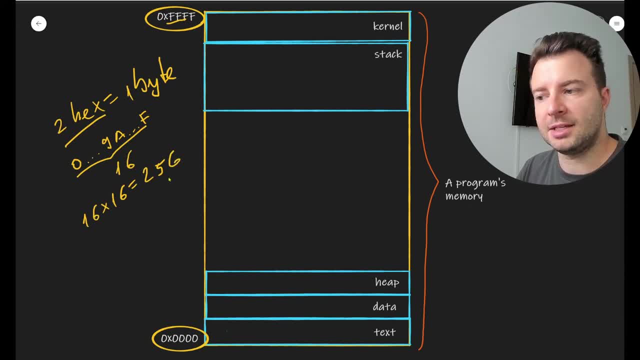 That's the maximum value of a byte, because a byte is eight bits. two to the power of eight is 256.. Right now, coming back here, let's see what all these memory regions are, And we're going to start with the least interesting ones. 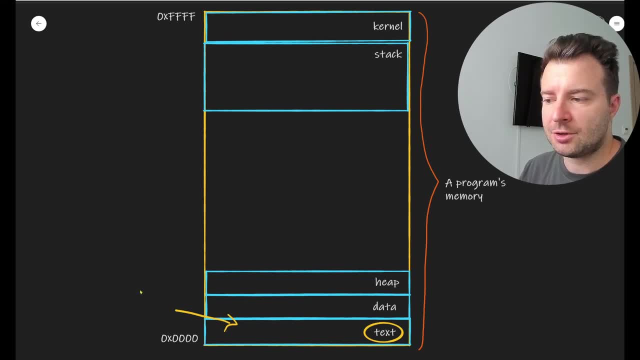 Like the text area. Now the text here is going to store the actual program code. Those are the actual program instructions And most of the time they're going to be read only So. we don't really care about those because we cannot change those. At the top we have the kernel area, which is not 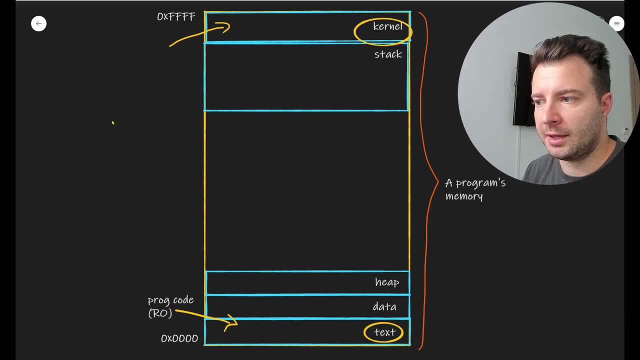 the operating systems kernel. But we are going to find in here stuff like the arguments that we use to launch the program and also some environment variables that the program might use. Then the data area stores variables- initialized variables, uninitialized variables doesn't matter, they're. 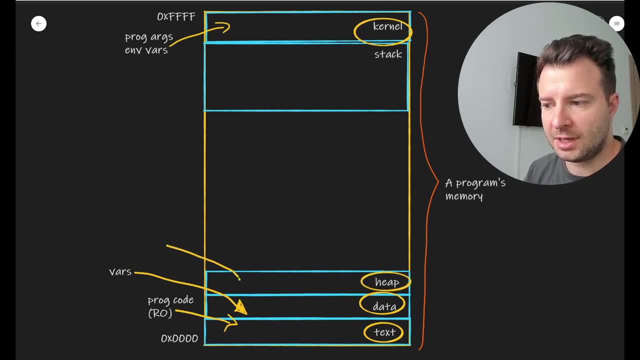 all here. Then we have the heap. Now the heap stores what I like to call the big stuff, That is, files that you load in memory: the document that you're currently editing in Word, for example, or the level that you're currently playing in a game- Anything that's not a variable or a simple data structure. 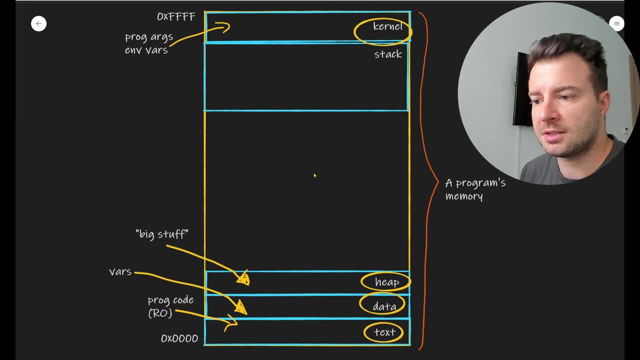 and needs to be loaded into memory and takes up a lot of space, is going to be stored here in the heap, And we're also going to find the global variables here as well. And we left the stack at the very end because this is where things get interesting. 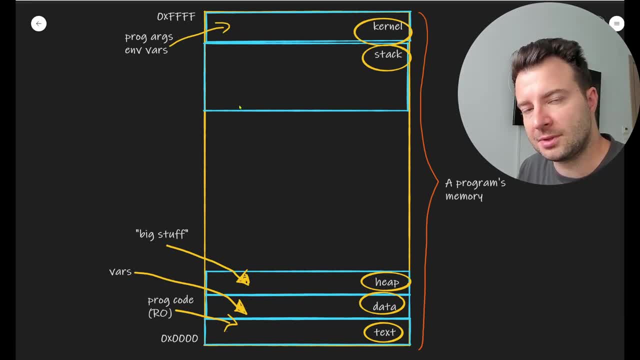 We're going to talk about the stack in just one second Now, before discussing about the stack, there's one more thing here that you should know. You've probably noticed that we have a big unpopulated area here in the middle. So what's this? What's this area Now? 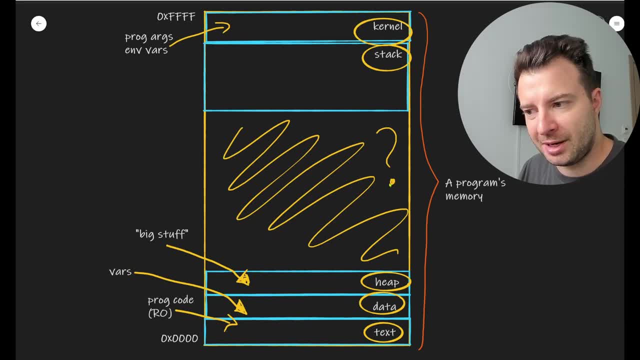 this data structure is, by default, empty, but we have two memory areas that are constantly competing for it from two different sides And, as you can guess just by looking at this picture, the first one here is going to be the stack and the second one 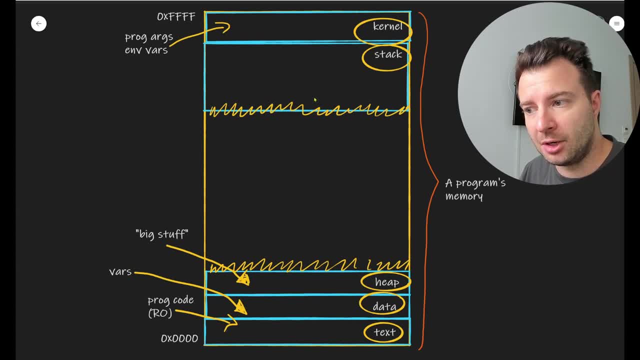 is going to be the heap, And that's because both the stack and the heap can grow when needed and they will start taking up space from this empty area in the middle. Now the heap is going to grow, of course, whenever you need more memory to load more stuff into it, like another document. 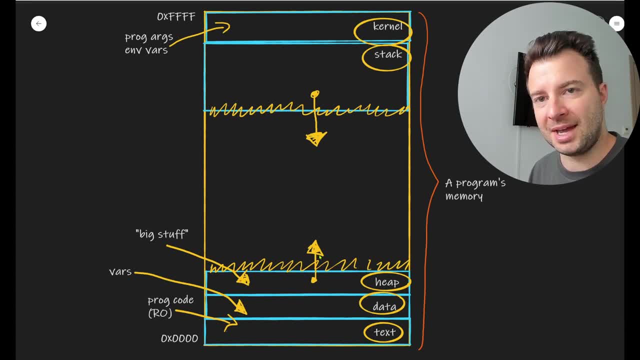 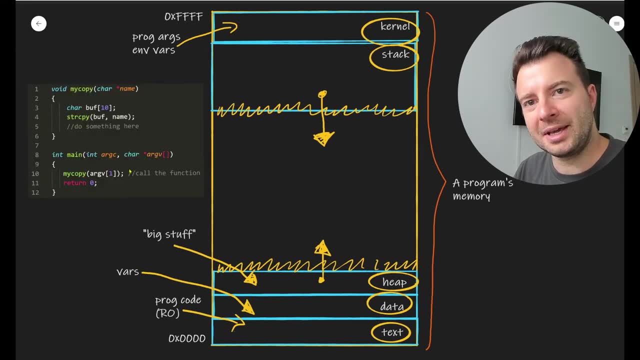 another PDF file, another level Now, in order to understand how the stack grows, and what exactly does a stack do, let's have a look at a very short piece of code Now, don't freak out. This is a simple C program, right here, which. 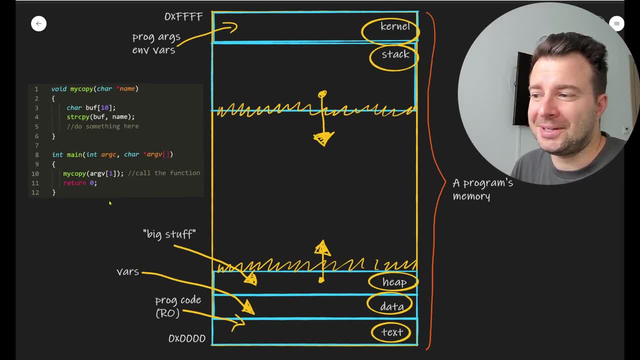 doesn't do much. It actually doesn't do anything, but you don't need to know C programming for the CISO Plus exam, but we need a very simple example like this just to exemplify and show you what happens when a buffer overflow occurs. Now this simple program here, like any other program. 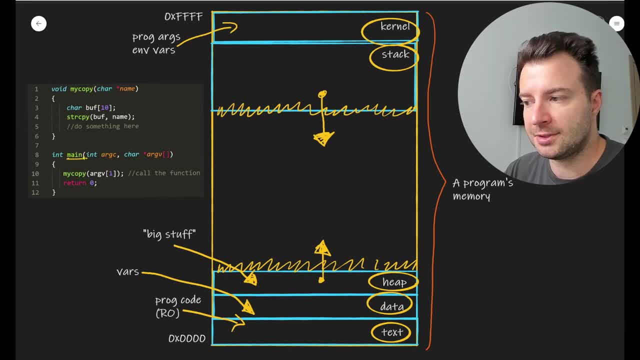 is going to start its execution with the main function. That's going to be the first function to be executed and the first instruction on line 10 is going to be a call to the myCopy function. Now the myCopy function also receives a call to the myCopy function, which is going to be a call to the myCopy function. 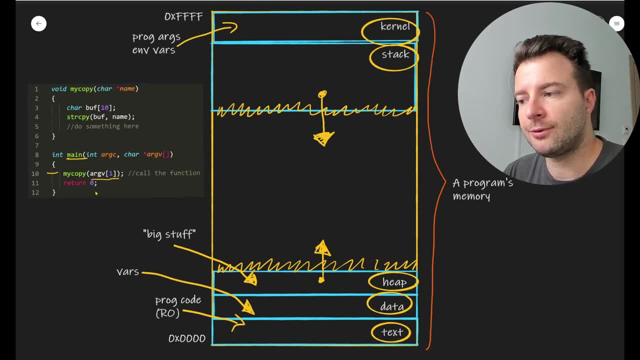 Now the myCopy function also receives an argument. This argv that you see right here is going to be the first argument that I provide to the program when I launch it. For example, if my program is called hello right and I write in the command line hello Andrew, then Andrew is going to be that. 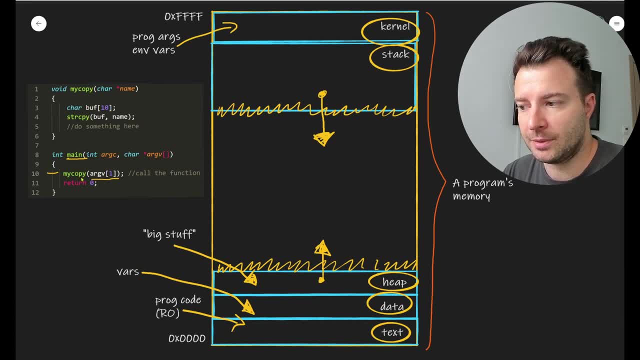 first argument: that gets passed to the myCopy function. And well, when the execution, the program execution, sees this function call, right here on line 10, the program is basically going to jump its execution and it's going to be a call to the myCopy function. And well, when the 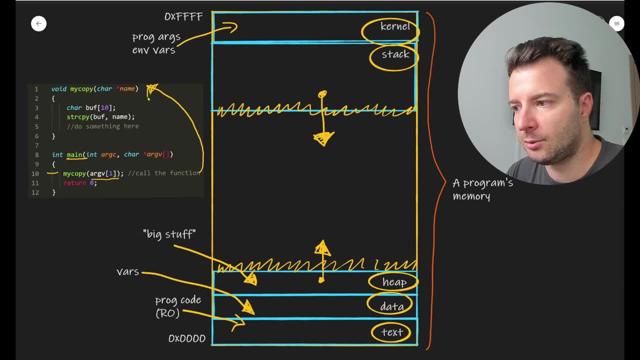 execution is called, it's going to start executing instructions one by one from this function right here until it reaches the end of the function, and then the execution comes back to the following instruction in my main program, just like you would expect whenever you call a. 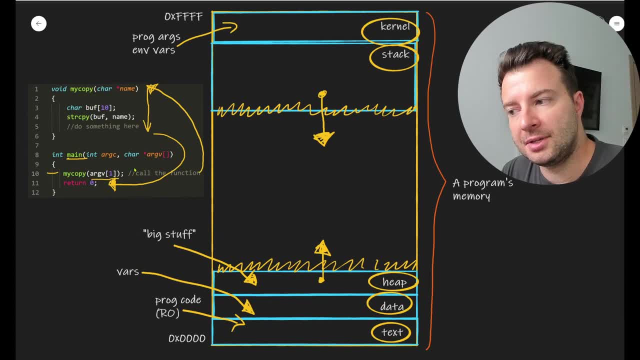 function in any programming language. Now this type of execution here is going to involve the stack. So before the program starts executing the myCopy function, it's going to store the following things on the stack. First, it's going to extend the stack. 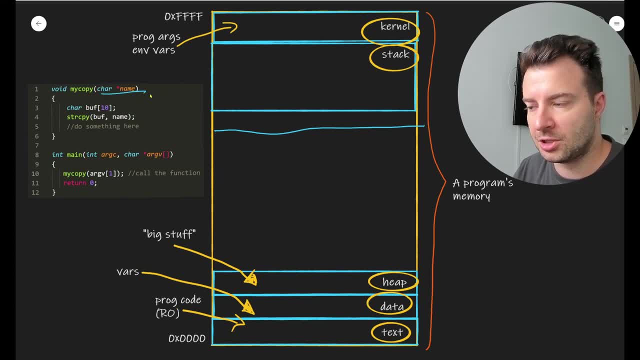 to make room to store the arguments of the my copy function, in this case the name parameter, and it's going to store it right here, all right. next thing that ends up in the stack is going to be another place allocated to store the return address for this function. now, why do we need a 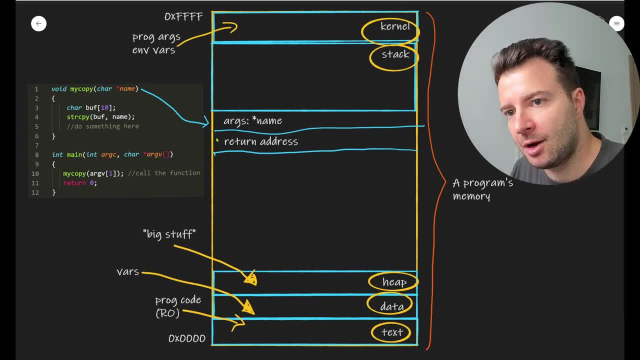 return address before the program needs to remember somehow to put a bookmark to the place where it previously was before it started executing this function. think of this just like the bookmark that you would use when you're reading a book and you want to just to perhaps peek a few pages ahead, or 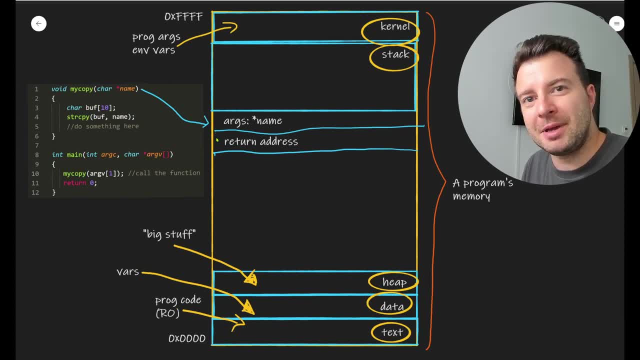 just look at the table of contents. you just use a finger or a paper bookmark just to mark the current page and then you look back or forward into some other location in that, in that book. right when you're done checking that outside info, you know exactly at what page you need to go back. 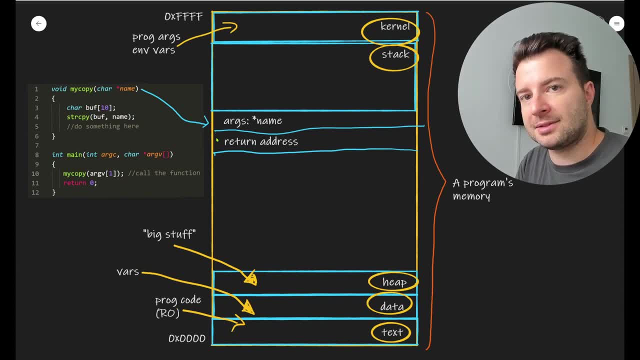 to where you were before you digress from the and access some other data. so that's exactly what happens with functions as well. the program execution actually left the main function to head over and execute the my copy function. so when my copy is done, the program needs to know where it's supposed to come back to. in our case, here would be. 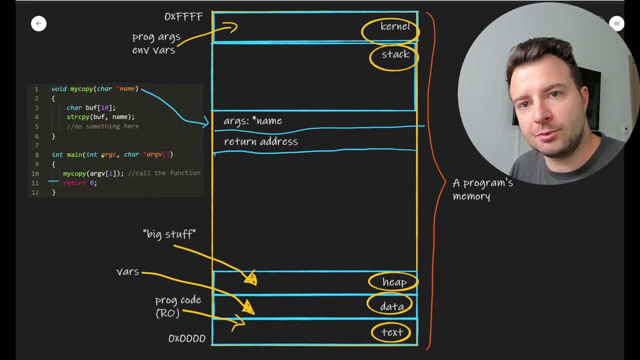 line number 11, which is actually the end of the main function as well. but that doesn't matter, right, it's good it could be any other additional instruction present in the main function. so the return address is going to be a memory address that points to the next line to be executed in your main program. and one more thing we're going. 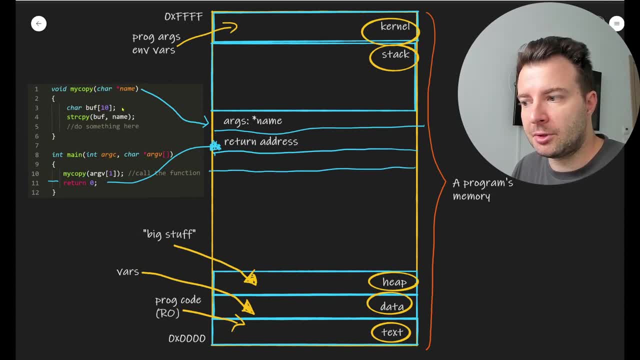 to also store on the stack. we're going to allocate more memory here and we're going to store any local variables or any variables that represent the current context of our function. so in this case, our buffer of 10 positions, our character buffer of 10 characters here is also going to be stored. 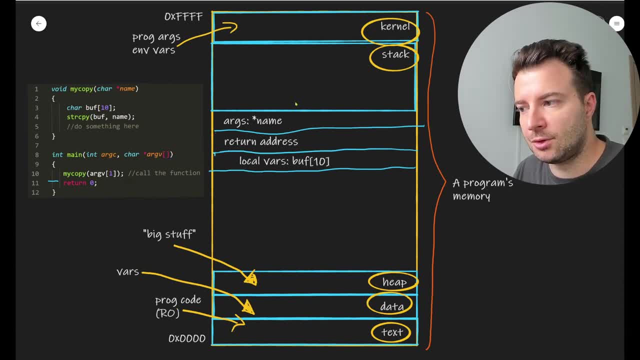 right here on the stack now, of course, when we're done executing the my copy function. all this information here is free, so we're going to store it right here on the stack and we're going to store it here for a while, but, btw, that's just for comfort later, now that we successfully got that back. 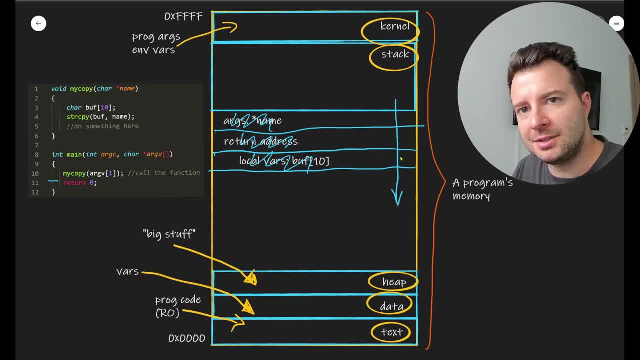 so now we just have to save it here. good, okay, structure that behaves just like a, let's say, a stack of plates. right, Let me see if I can draw a couple of plates here. Just imagine that these are plates And the idea of a stack is that. 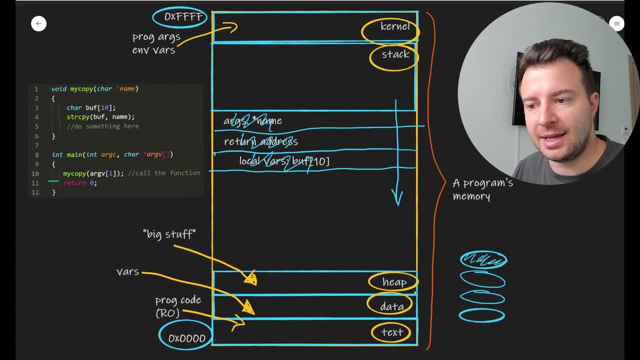 you can only access the topmost element in that stack, the one right here. We actually have a couple of operations, and the most important ones are the operation of putting something on the stack, and this one is called a push. Another operation is removing something from a stack. 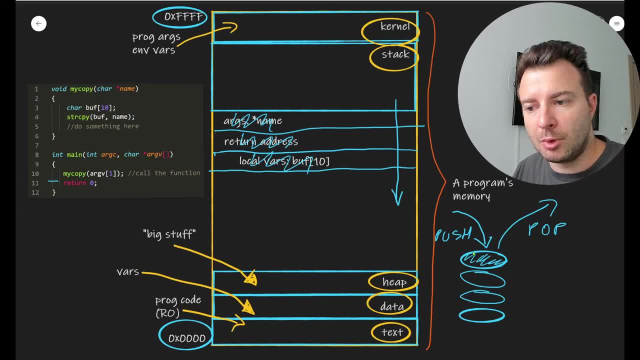 which is called a pop, And, as you can see, we can only work with the topmost element. And of course there is another type of operation here which is called peak, which allows us to just read the first element without removing it. But the main idea here is that in a stack data structure, 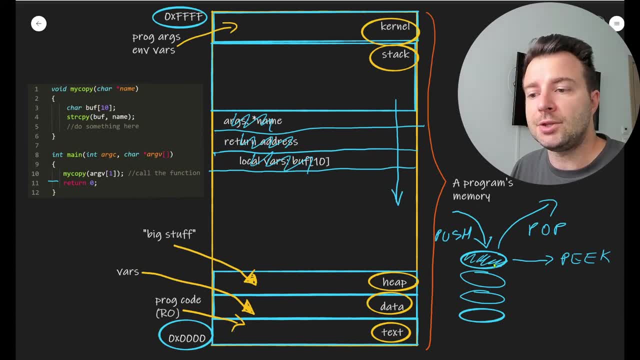 which is a very widely implemented data structure. in programming you can only access the topmost element at any single time. So in our case here, our topmost element would basically be our local variables. That would be our buffer. Now let's go back to the code for just a second here and look at what this my copy. 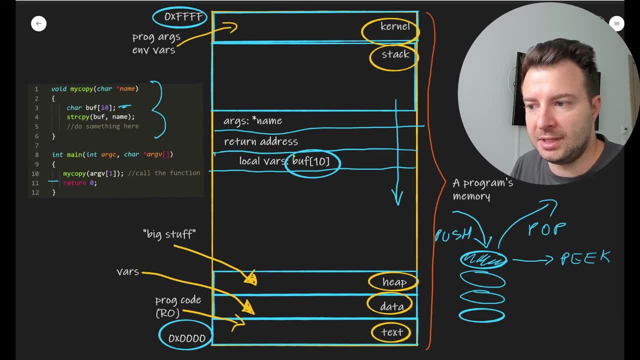 function actually does, You can see. it allocates a buffer right here, which we've seen- that it ends up on the stack. And then we have a simple function call Another function. this one is built in into the standard library of C or C++ And what it does is actually copies one string into 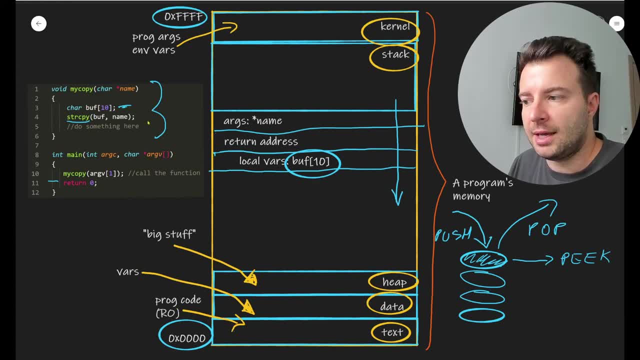 another, a string of characters into another. And this string copy here is considered to be an unsafe function because it receives only two parameters. First one is the buffer. That's the destination. Where do we want to copy that content to? And then 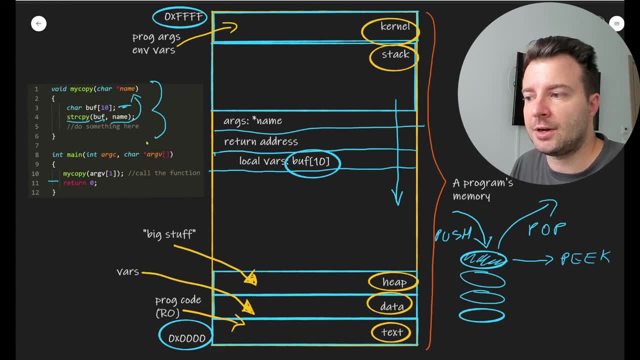 the name, which is actually the variable that you see the function receives right here at the top as an argument. that's the source of the data. So, basically, what this function does is reads the contents in this string of characters called name until it reaches a zero value, a null, terminating. 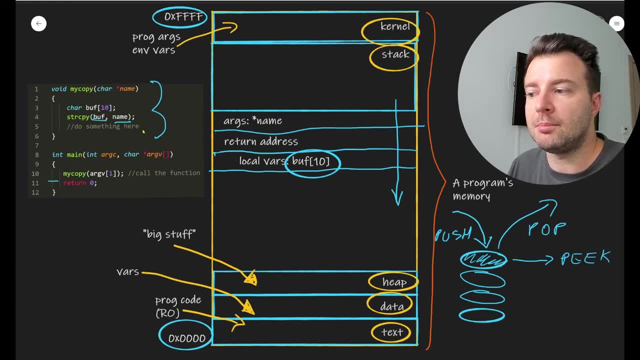 value and then puts its contents into this buffer, which is pre-allocated right here. Now, of course, if name here is less than the 10 characters that we've allocated for this buffer, everything would be just fine, right, We don't have any overflow happening here. The buffer can. 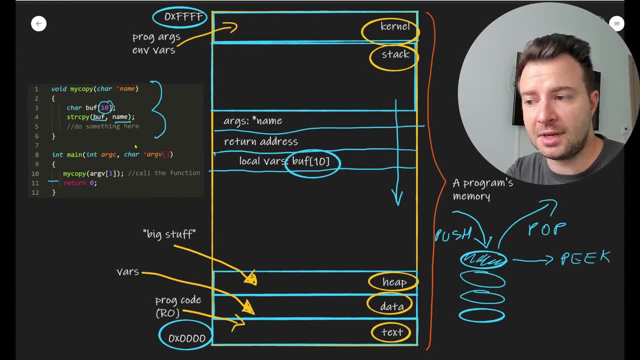 hold as much data as we give it, And inside of the stack, things would probably look something like this: Now, assuming that the argument that we've launched this program with is something like Andrew, then this string Andrew right here is going to end up in this allocated space inside. 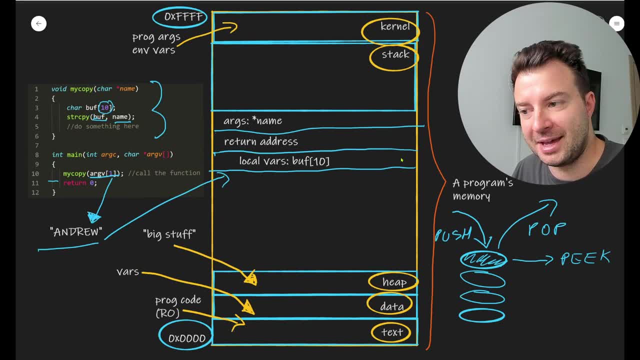 of the stack. And another weird thing, another weird behavior of the stack is that, even though it grows from high values to low values, well, the way memory actually gets allocated is from low values to high values. So what we're going to do here is actually not store Andrew like this, but instead we're going 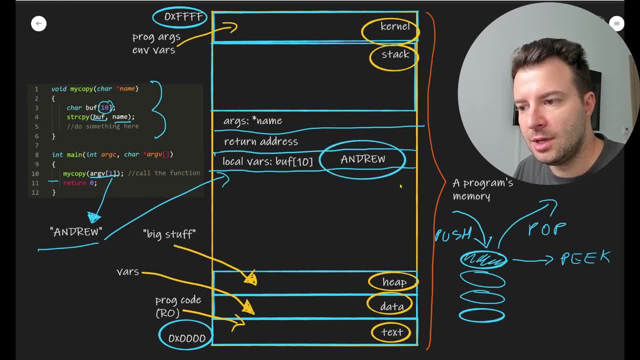 to store it in reverse order so that we can go from lower values to higher values. So we're going to basically write it from right to left, kind of like this: This word over there, word right here now. remember, this buffer only has 10 positions, so we can only store at most. 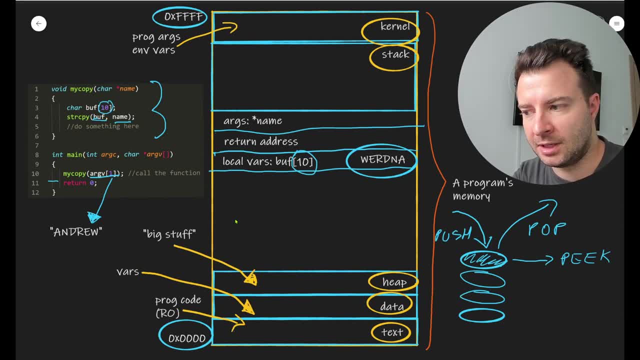 10 characters in here. so what happens if andrew suddenly becomes andrew one, two, three, four, just like this? well, it's going to end up in the stack as four, three, two, one word now. okay, we still have a valid buffer here. but what happens if andrew one, two, three, four actually becomes andrew one? 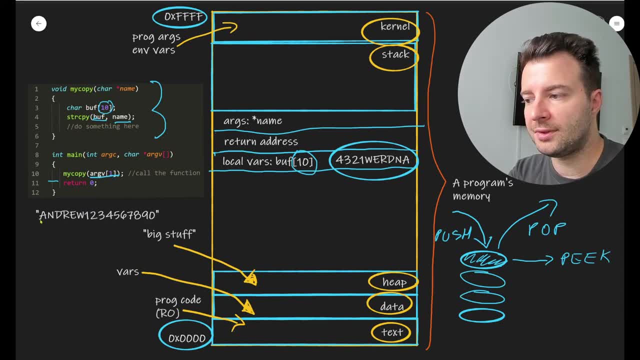 two, three, four, five, six, seven, eight, nine, zero. what happens with this string when we try to give it to the string copy function? well, remember when i said that the string copy function right here is considered to be unsafe? well, that's simply because, as you can see, it receives two arguments. 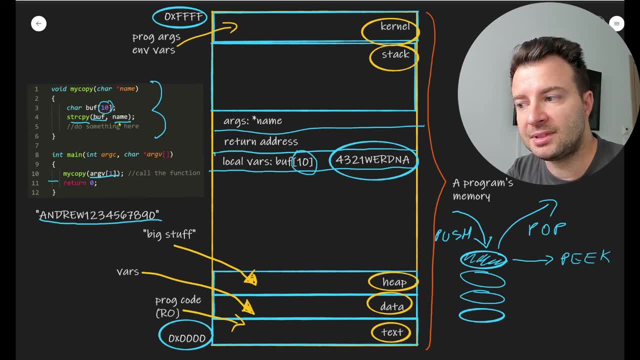 the one is the- uh, the destination and the one is the source. but there's no argument saying how much should i copy from this string copy function from the source to make sure that i'm not going to overflow the buffer in the destination. and if you think about the fact that, well, the program is is going to take care of this, the operating system. 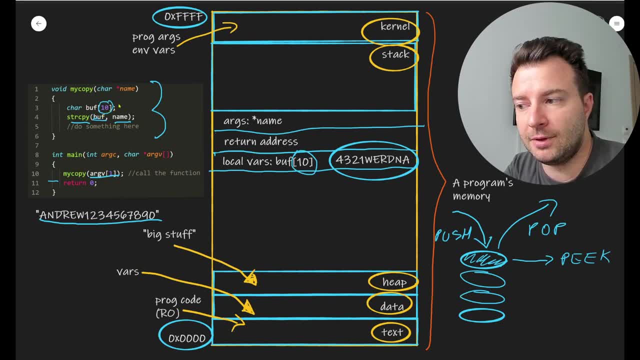 is going to take care of this. i mean, the operating system sees that i only have 10 values here. how could it attempt to write beyond those values? well, that's another discussion here. but actually the buff and name parameters that we have in here don't contain the entire string pre-allocated. 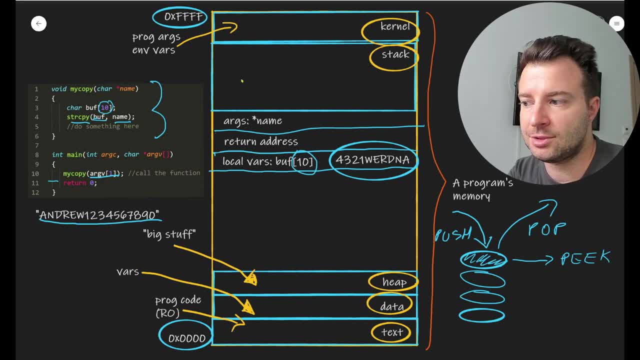 string. these are just pointers to the beginning of the string. so basically the string copy here what it does. it says: start copying from the name location to the buffer location. as long as you find something in the name location, there's no stopping it. right, there's nothing to tell it. 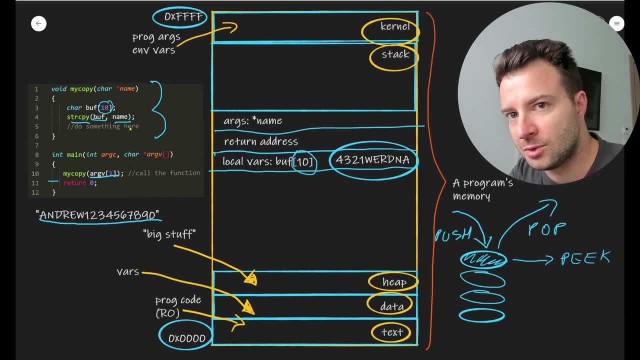 to stop after 10 characters, and this is where we're going to cause a buffer overflow. now, a buffer overflow like this is going to happen in the in the stack is going to occur in the in the in the stack is going to occur in the in the in the stack is going to occur in the. 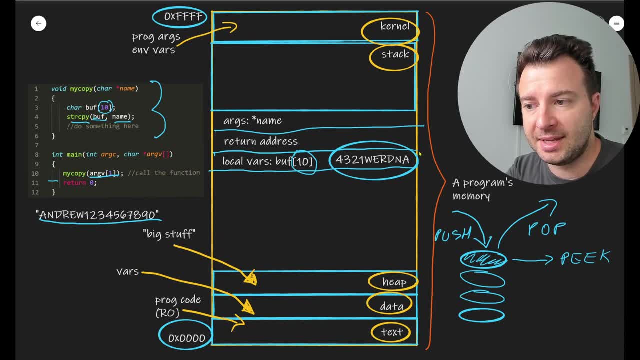 in the stack in a very nasty way. that's because the space that we just allocated in the stack for this buffer has depleted, so there's no way for me to keep adding here five and six and seven and so on. no, what's gonna happen is it's going to continue writing onto the next available address. 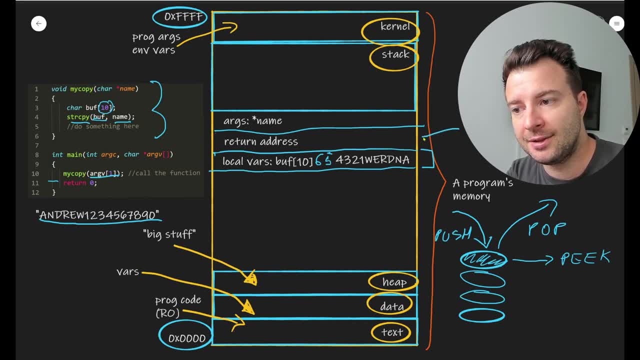 inside of the stack and which one is the next available address? well, this field right here, the return address, and it's going to start overwriting the return address with the rest of the content that i've provided in the stack, and i'm going to start overwriting the return address with the rest. 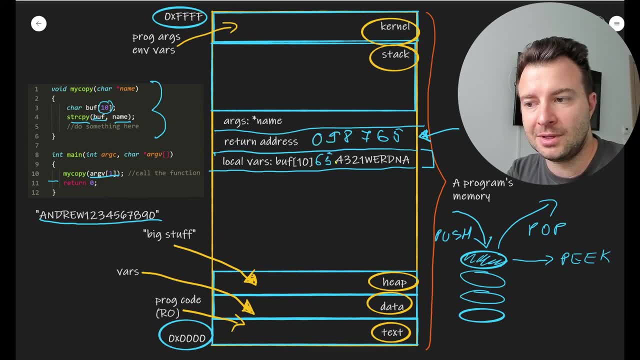 of the content that i've provided inside of my buffer. now, what's going to happen now? the problem is that whenever the my copy function finishes execution, the program is going to try to read this return address right here to figure out where to jump its execution. ideally, this was supposed to. 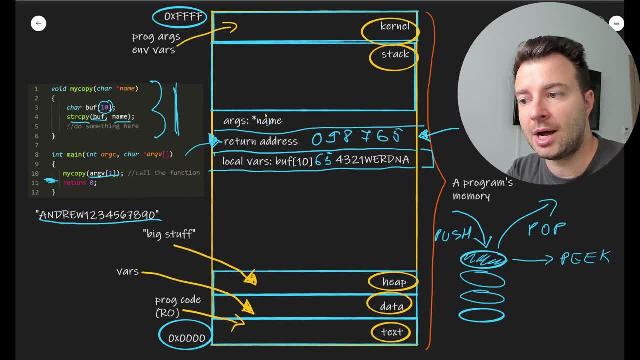 hold line number 11 in our code right now. i've just overwritten it with some arbitrary values. now, in most situations, if this happens accidentally, this is going to end up as a segmentation fault. so that's going to be an error which is going to crash your program, because 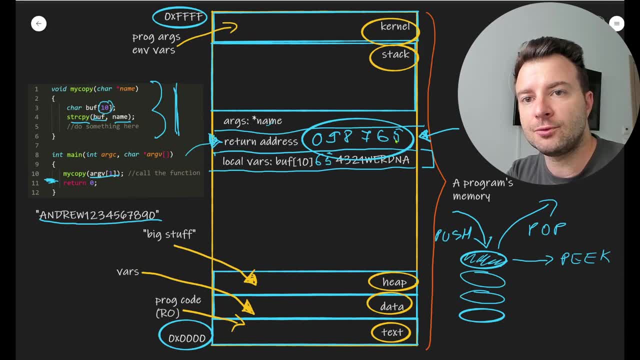 there's probably not going to be a valid address like this for the program to jump to. but imagine that you are an attacker. if you are an attacker, then you can actually craft the contents of this buffer right here to make sure that the end of it includes the exact return address that you 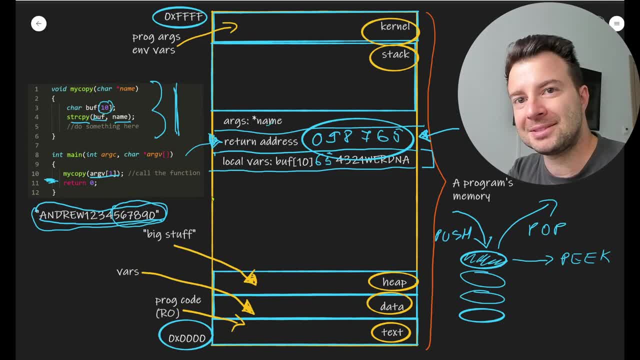 want your program to read whenever it exits its current function. now you're basically telling the program, through a buffer overflow, go ahead and execute some other piece of code, some other type of code that i've provided you, and that's a very dangerous type of attack because you're basically 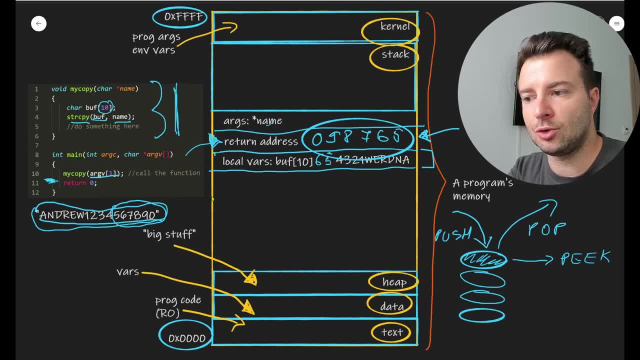 interfering with the normal program execution. you're telling it: just ignore your normal code, start executing my code, and this is how you take over. you take control of a remote system. you can tell that system well, instead of executing your own functions, execute a reverse shell for me, or. 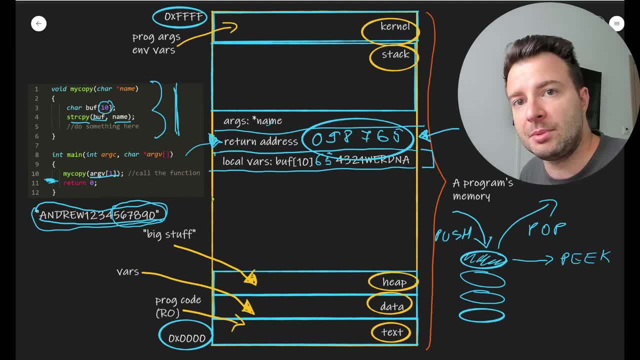 a denial of service, attack for me or execute anything on my behalf, which means that i currently have access to that machine. i can control that machine, and that machine has been breached and is under the attacker's control. complicated stuff, i know, but it happens and it's actually the most. 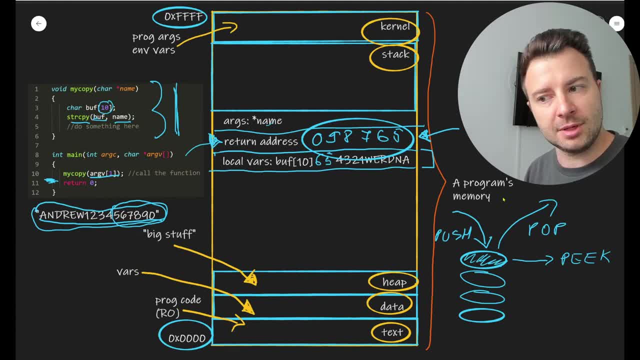 common type of exploit. unchecked boundaries, unchecked buffers that can be overflown can be easily hacked using examples very similar to the one that i've just given you here, so that a can just send a valid request, can be over http, over the network, it, sometimes it can even be an. 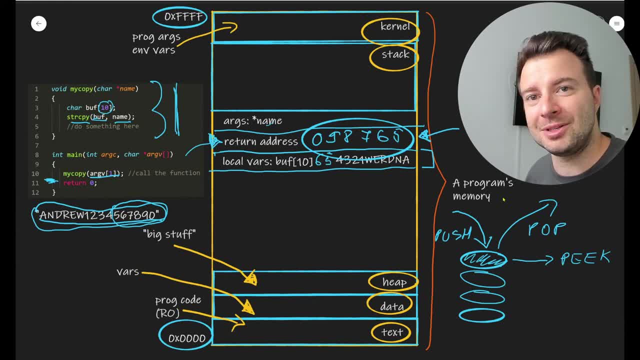 email or just a file that you you trick someone into opening it, and all that file is going to provide an input that's going to overflow a certain buffer which the attacker knows, that is going to allow him or her to overwrite a return address and to cause that program to jump its. 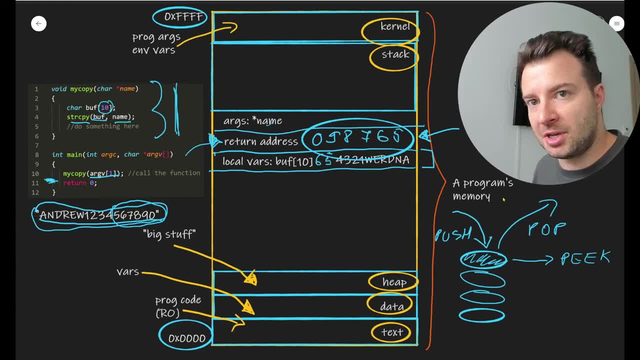 execution to some different piece of code provided by the attacker. now, most most likely, that additional piece of code, that malware code that you vince, the, the program to execute instead of its own code, is also going to be provided through that buffer overflow as well, so the, the attacker, can actually do something like this. i mean, you don't? 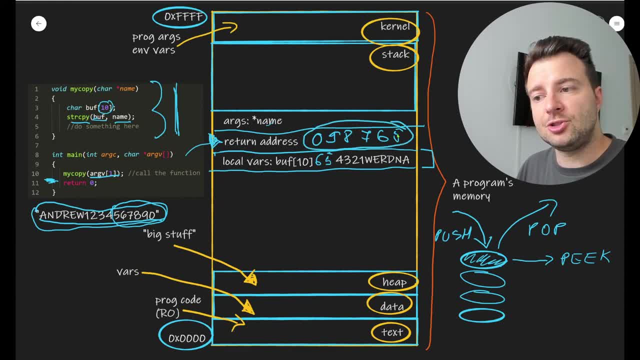 even need to jump that far. you can just take this crafted jump address right here and tell it. you know, jump maybe a couple of positions downstairs in the stack and start executing code from there, because this, this area right here, is most likely already part of that buffer that was provided. 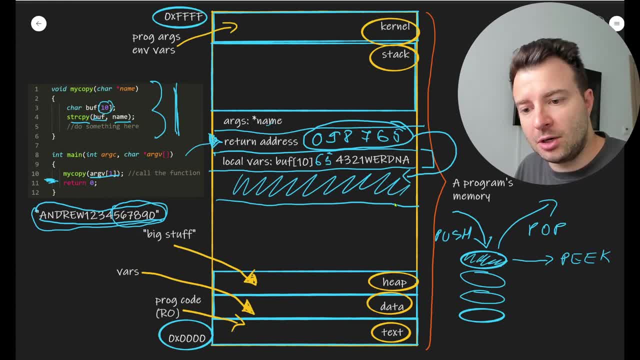 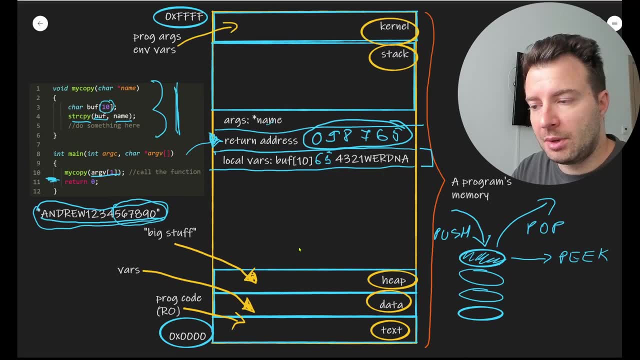 as part of the overflow attack, so you're basically providing the code as well as the jump instruction to that code to be executed on your behalf. it's it's that easy and all. in many cases, the memory is randomized, so perhaps the attacker doesn't know exactly where to jump because it 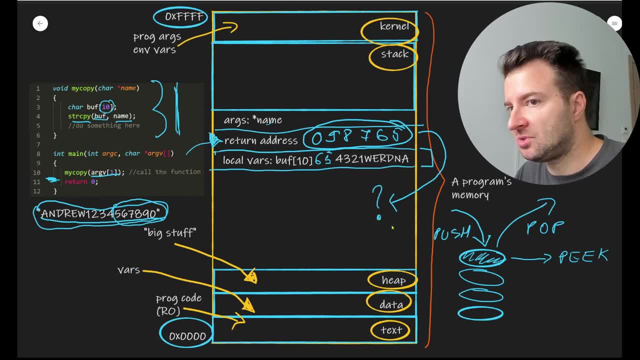 doesn't know exactly where its buffer is going to end up in memory. it doesn't matter. we have a solution for this as well. if we don't know exactly where to jump, that's okay. we just fill in as much as possible with a huge amount of memory, and that's what we're going to do in this case. we're going to 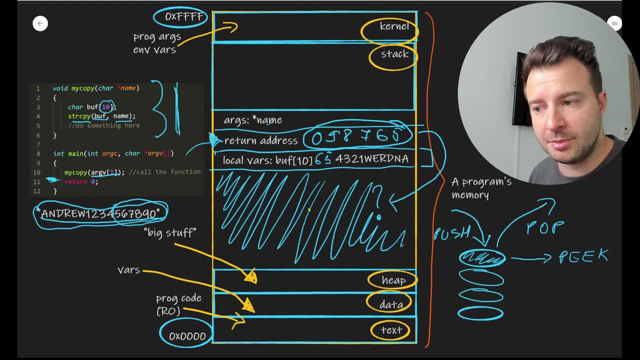 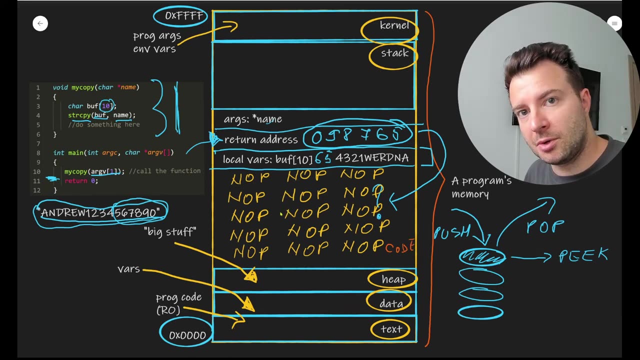 do a huge buffer in here. we take up all the memory, or as much as possible, and we fill it with do nothing instructions, which are also called knobs or no operations in assembly language, and at the very end we put the actual malware code right here. so we don't know exactly where our code is going. 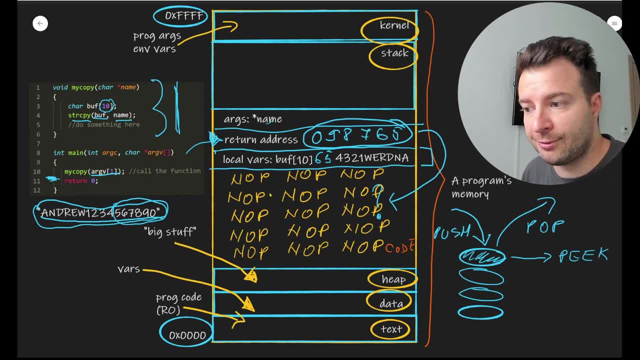 to end up or where our code is supposed to jump. to execute it, we just fill the memory with knob instructions like these and whenever we jump that code, you just have to hit some position inside of this knob area, doesn't matter where. when it hits a knob instruction, it just moves on to the next and 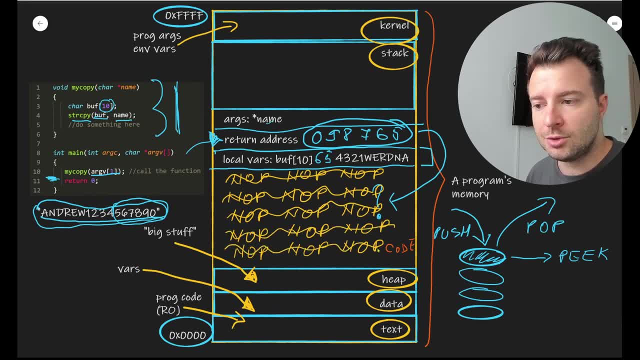 then to the next, and keeps going, and keeps going until it reaches and executes our malicious code right here. and this, by the way, is called a knob sled, because the code basically slides down through all these instructions, just ignoring them, just like a sled would would go downhill until it. 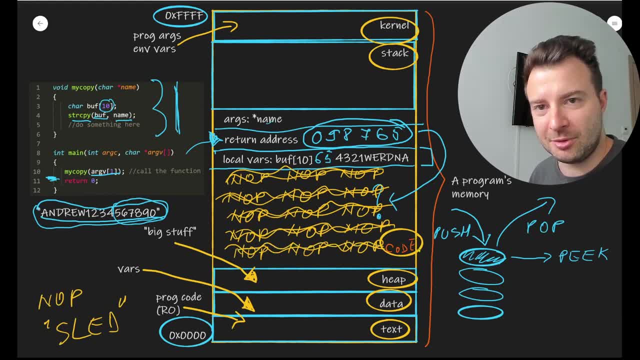 reaches the executable code. that's the the bottom of the hill. and, by the way, if this happens inside of a stack, i believe it's obvious enough that we're going to call this a stack overflow. there are also heap overflows and other types of overflow, but for the exam at least, this should be enough right now, and well at least. 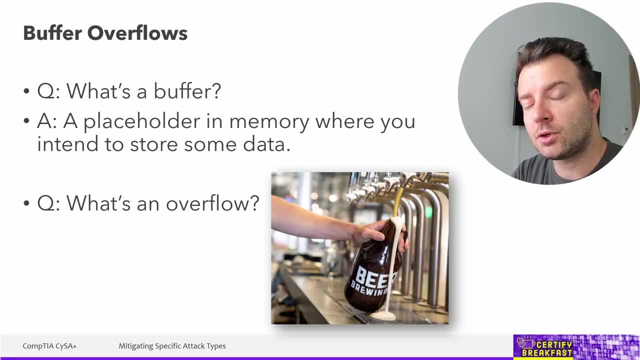 now you know where the name of the website stack overflow comes from. a buffer overflow exploits can be very dangerous because they can either allow the attacker to inject their own code or to perform privilege escalation, basically- or allow the attacker to read restricted areas from the memory, like regions that store secret keys, passwords and session ids for 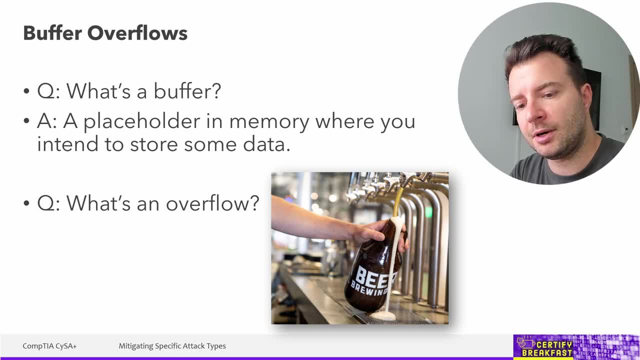 example, one thing to keep in mind is that if you're using a buffer overflow to perform privilege escalation, you can only escalate the privileges up to the privileges that the application is using to run, because you're basically tricking the application into running your own code. so your 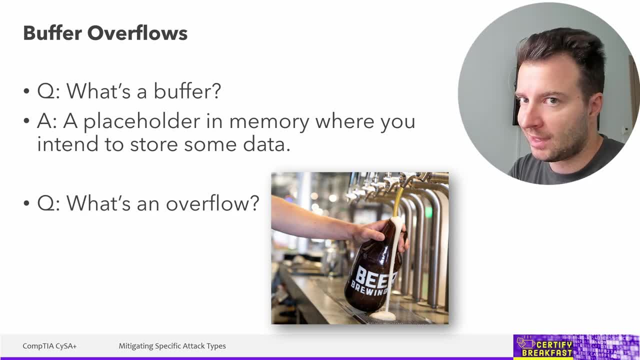 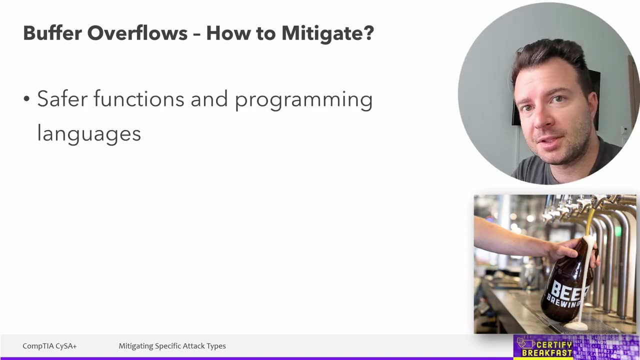 own code is going to run with the permissions that the application currently has. now you've got not going to instantly become root, but you will become a valid user on that machine, all right. so buffer overflows are bad, are dangerous. how do we prevent them from happening now? first method would be, of course, write better code, right. 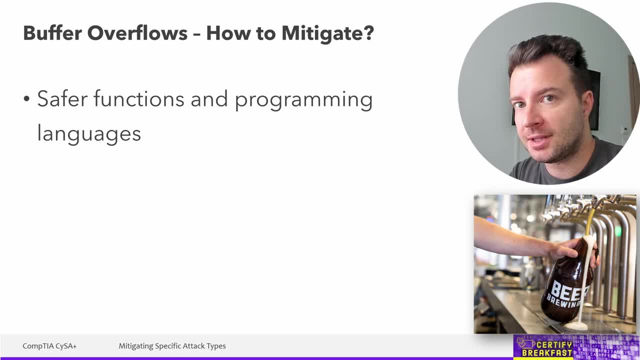 safer code. there are functions that are safer than others that perform boundary checking, especially in situations where you're copying information from one location to another. and secondly, we also have different programming languages that behave differently and they manage memory. for example, c or c plus plus are going to leave the memory management. 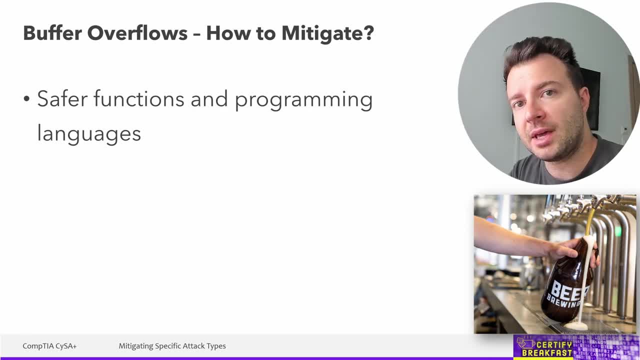 mostly into the programmer's hands now, on the other hand, we have higher level applications like dot net or java or c sharp or any application written in dot net, for example, that have a more strict control over the, the input that you're providing, and their internal functions by default. 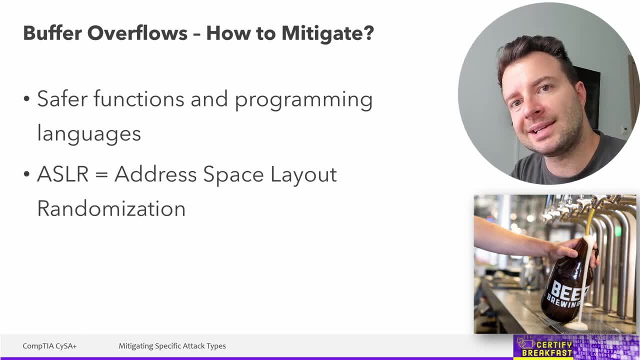 are safer now. the second one is called aslr, that's, address space layout randomization, which is of confusing the attacker by randomly positioning those, those memory blocks like the stack, the heap, the, the libraries that get loaded in the memory all over the place, which makes it harder or even 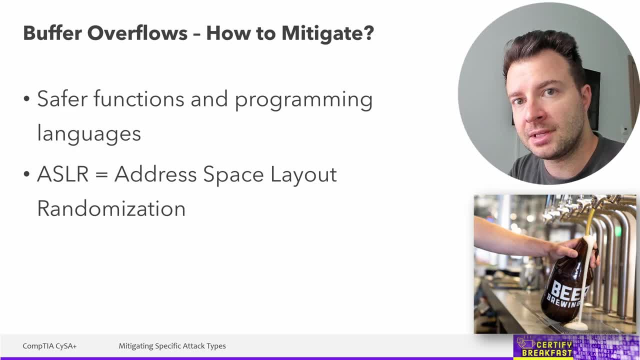 impossible for an attacker to determine at which address his or her malicious code is located, so they might not be able to execute it, even though they might be able to inject it. the stack canary is an interesting one. it's a very small integer value that it's placed on the stack right before. 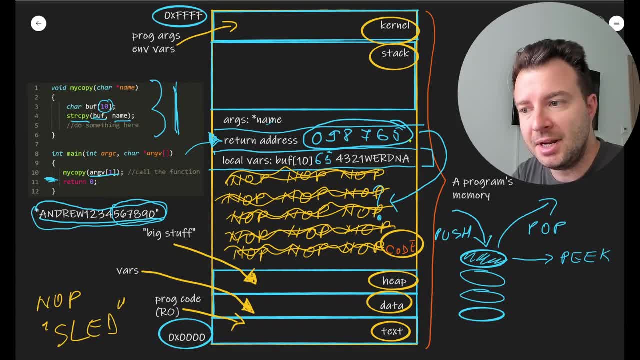 the return value of a function, all right. so in our example right here, we're going to add a small value right here before the return address. remember, we're writing this from right to left and this one, let's say, it's 42, right here now. now we monitor for this value. so if a buffer grows, 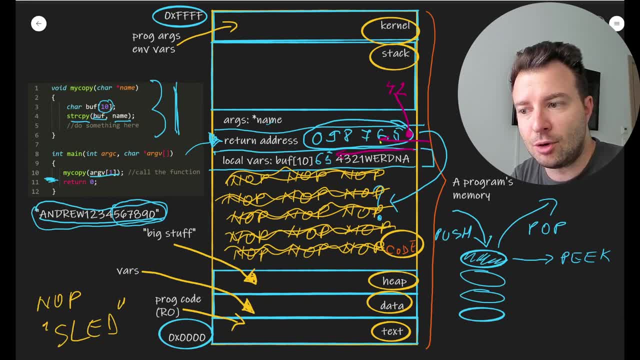 beyond its intended intended size and start overwriting this value right here now. if we lose it, then we know that a buffer overflow has happened and that we're screwed right. so that's a stack canary. that's a just a value that you're monitoring in order to 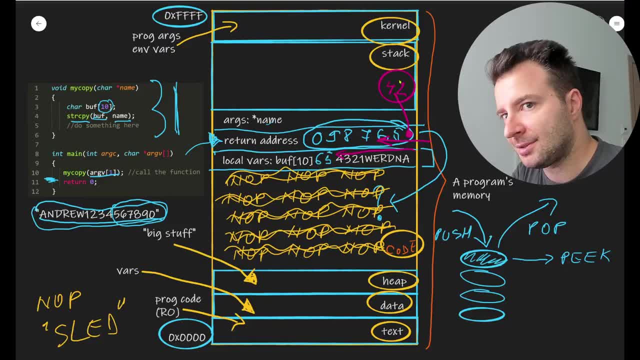 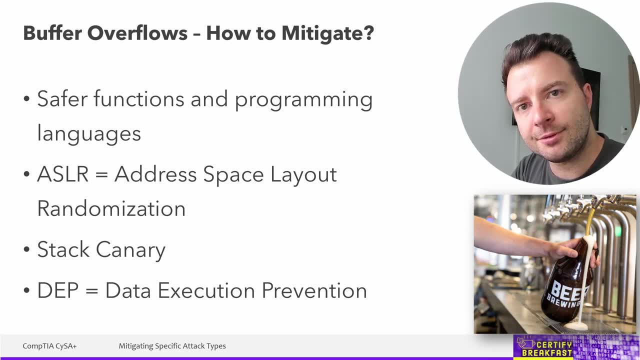 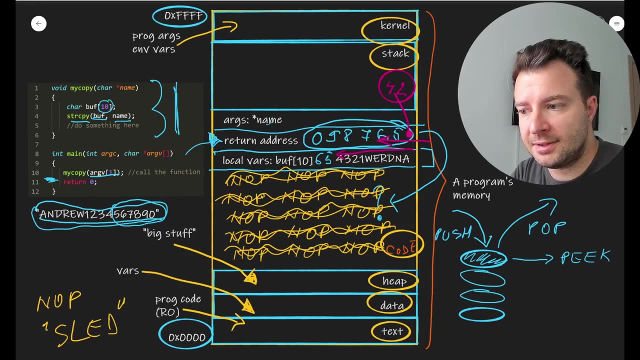 figure out if- and stack overflow- it might be happening or not. finally, we have deb, that's data execution prevention, which is available only on windows and it basically marks specific memory regions as non-executable. so in our example, we could tell the operating system that this entire space right here reserved for the stack is non-executable. so it doesn't matter if somebody 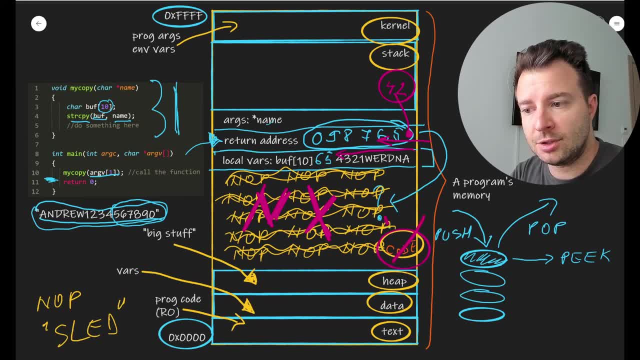 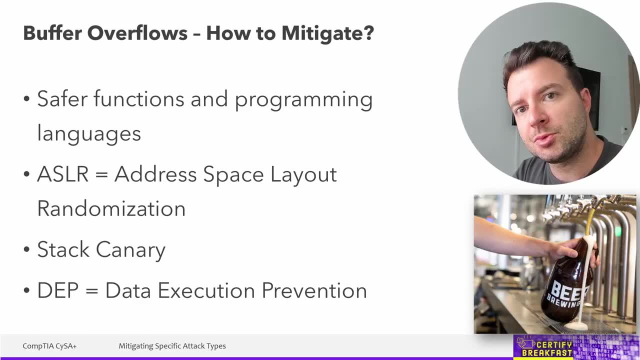 added their own code in here. it's never going to be executed because the operating system doesn't allow you to execute code from this location. so those are pretty much the main ways in which we can protect against buffer overflows. of course, we start with input validation. make sure you validate. 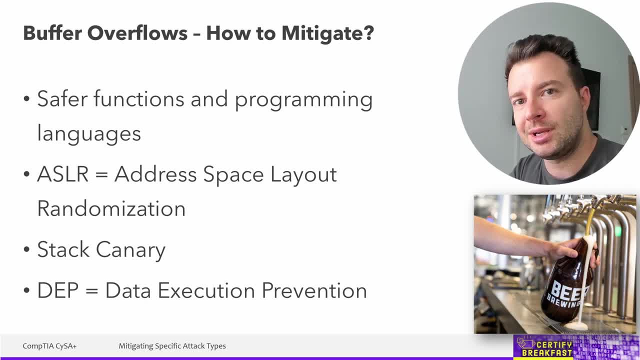 your inputs, so that you won't even reach that situation where you have to worry about what would happen if a buffer overflow occurs. and of course we have additional methods. for example, amd has something similar to data execution prevention as well, but of course we don't have to. 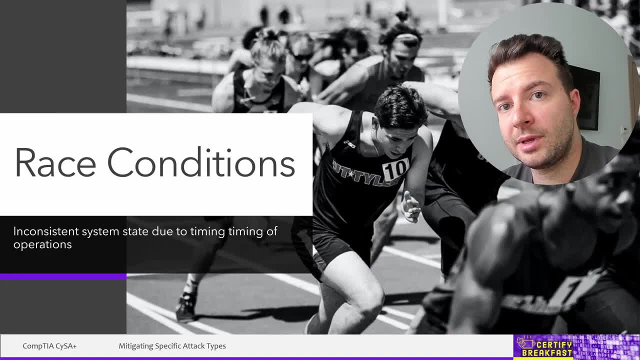 well, but for now this should be more than enough. next up we have race conditions. this is a design flaw, a coding flaw that allows a system to reach an inconsistent state simply because of the timing of its allowed operations. now this might not sound like much, but computers are designed to. 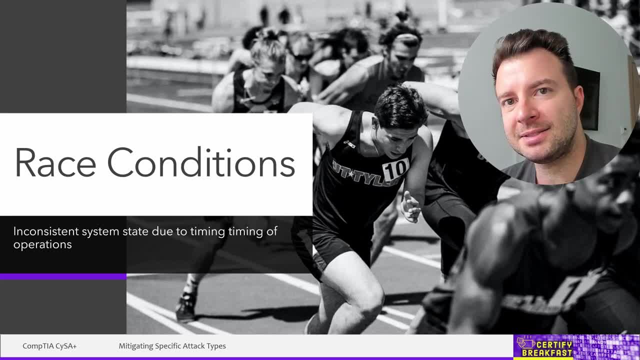 be predictable, deterministic. so having a sequence of operations that you cannot exactly predict what the outcome is going to be- well, that's really bad for computing. an example of this would be a situation where multiple threads attempt to write data at the same memory location at the same time. you cannot know for sure what the end result is going to be. which one is going to. 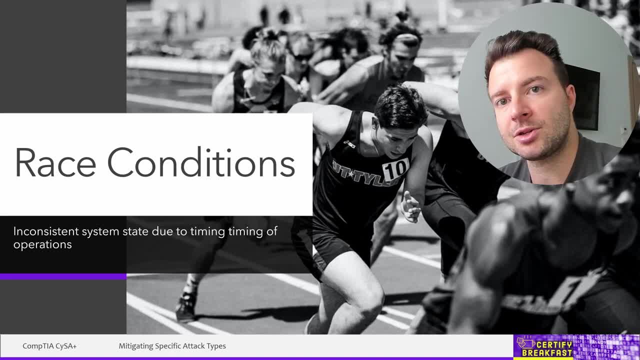 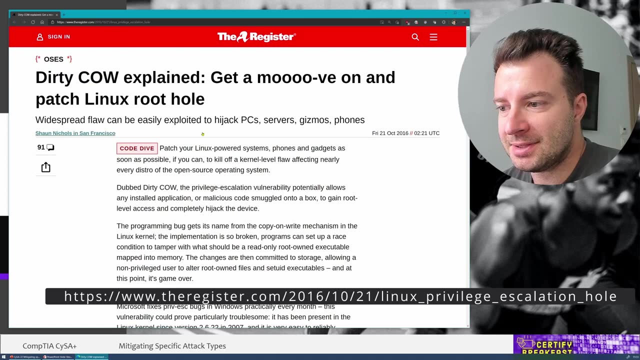 manage to write that data last, so which one is going to actually have a chance to store the data at that location? and the problem is that these race conditions can sometimes be exploited by attackers. a well-known example of such a vulnerability is was called dirty cow somewhere back in 2016. it. 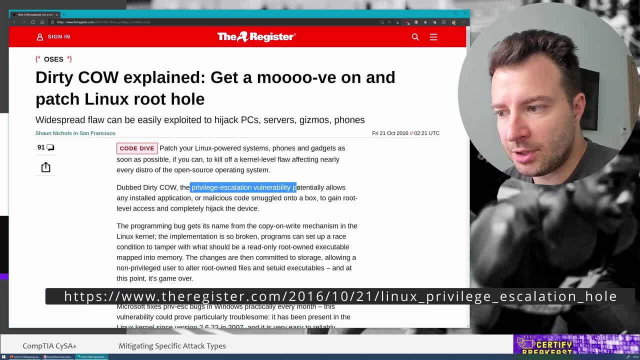 was identified. it's a privilege escalation vulnerability that can allow any application or malicious code to gain root level access and completely hijack the device. how scary is this? and the name comes from the copy on write mechanism. you can look it up if you want to. but very badly implemented so programs can set up a race condition. 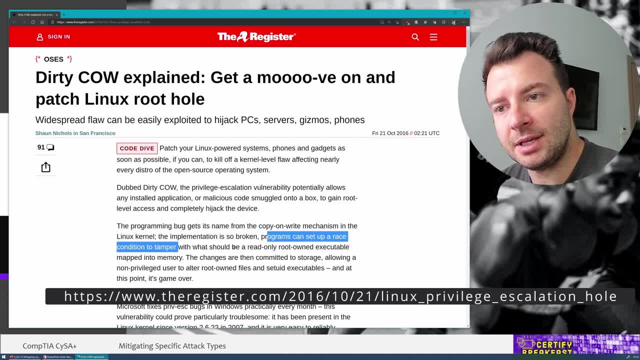 to modify a code that can be used to modify a code that can be used to modify a code that can be used to modify what should be a read-only root-owned executable. so basically, a non-root user can change root-owned executable files on any machine. so that's the definition of privilege escalation, what's even? 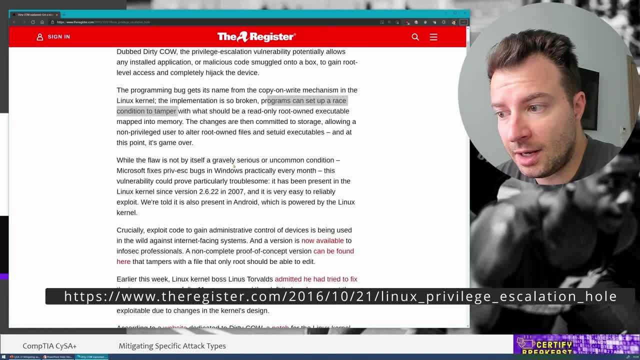 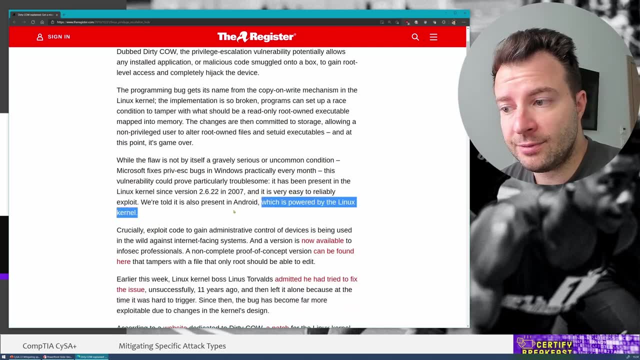 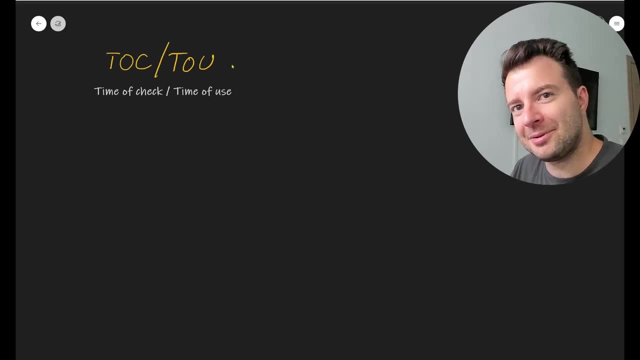 worse is that sometimes these vulnerabilities end up completely unnoticed. so this one was actually present in the linux kernel since 2007 and most likely it affected android devices as well, because they're also based on the linux kernel. now it's specifically interesting and even commonly encountered in the linux kernel, so this one was actually present in the linux kernel. 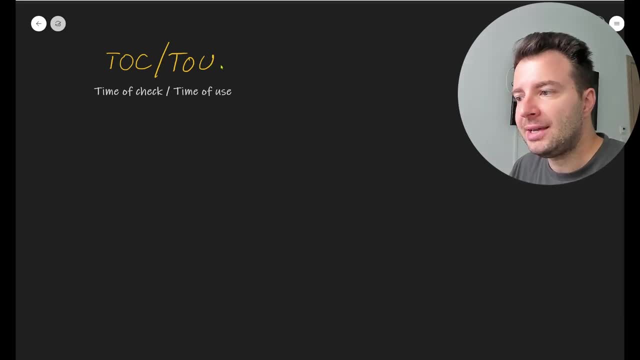 so this one was actually present in the linux kernel. so this one was actually present in the linux kernel. vulnerability that relies on a race condition is the time of check. time of use. vulnerability which is abbreviated like this, and it happens when programs try to modify a resource or a memory. 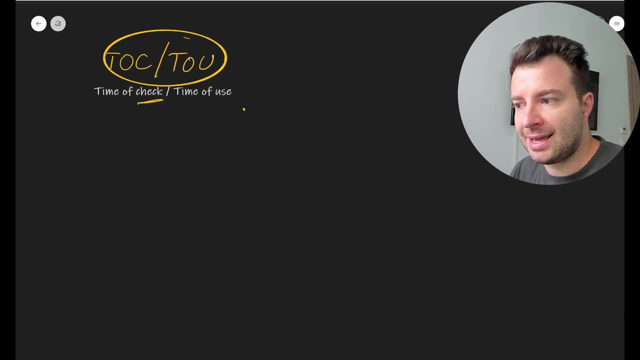 address, but they check that memory address and then modify it in two different, distinct operations. why does this matter? well, let me give you an example. so let's assume that we have two atms right- atm1 here- and atm2 right, atm2 right here- and let's draw a timeline right here in the middle. so that's this axis here. 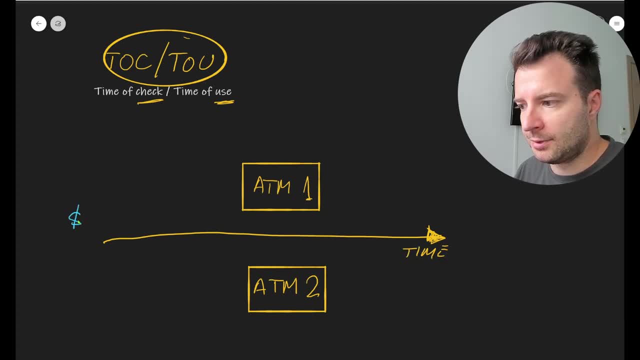 is going to be time and we also have a bank account with a hundred dollars. now let's assume we have two people with two credit cards that point to the same bank account and they both want to withdraw that hundred dollars at the same time. this is one scenario that could happen. the first: 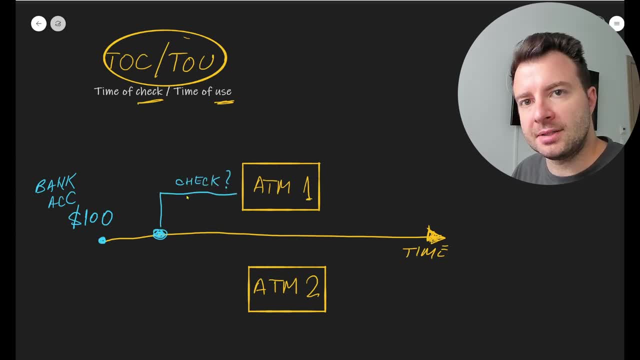 atm right here is going to check how much money is inside that account, and it's going to receive an answer that there are one hundred dollars available. immediately after that, there is a second atm right here is going to ask for the same thing and of course, it's going to receive a. 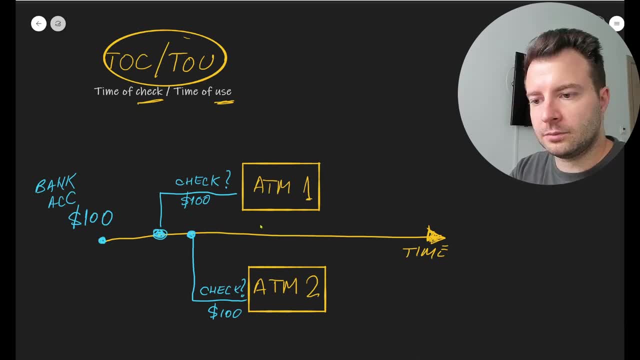 positive answer. the account has one hundred dollars. now the first atm tries to withdraw the hundred dollars that it was told that is available inside of the account and the second atm was also told that there are a hundred dollars available, so it's also going to try to withdraw that same amount. the 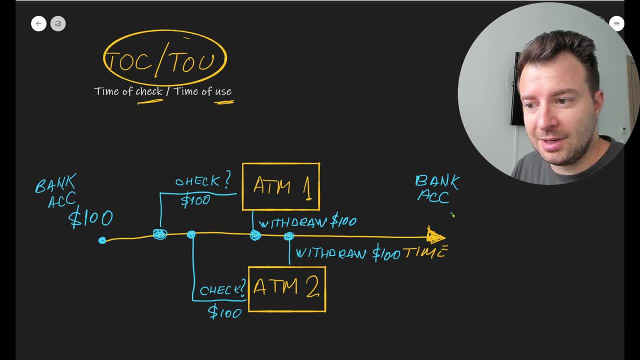 end result? well, we might end up with a bank account that is going to withdraw that same amount and the second, atm, is going to withdraw the same amount, because of the fact that we are going to withdraw 100 of the 100 dollars that we have from the bank account that currently has minus 100. now with real 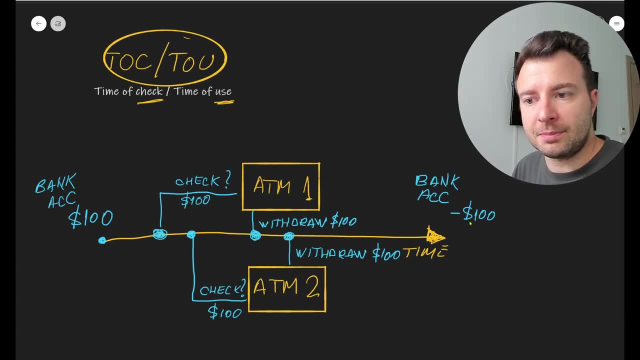 life banking. of course, there's no point in trying to do this, but in a badly designed software, this is a type of situation that can happen quite often and can lead to corrupted execution, to crashing programs and also to vulnerabilities that can be exploited. the problem here is actually the fact. 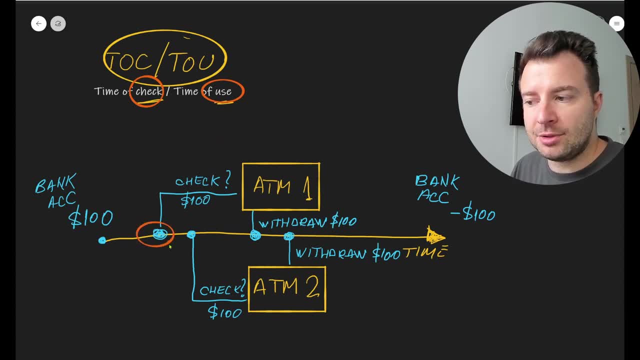 that we failed to connect these two operations, the check operations and the use operation. so when the first atm checked the amount of money that was collected, we can find out how much money it was of dollars inside of that bank account. it should have also executed the withdrawal at the same time. 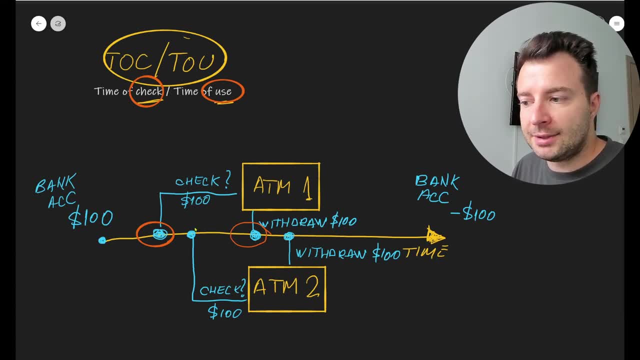 or at least in the same atomic operation, so that the other check here would not be able to happen at the same time and maybe misrepresent the state of the bank account to a different ATM at the bottom. So what's the solution for race conditions and time of check time abuse vulnerabilities like 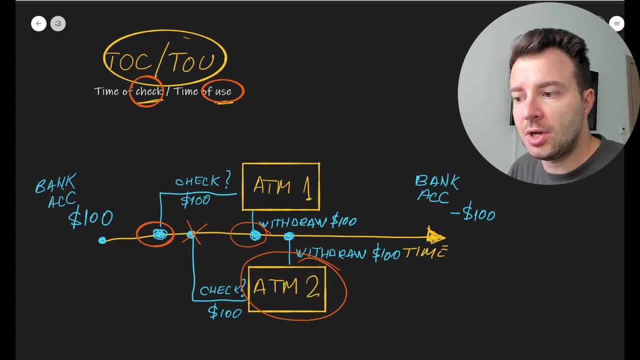 this. Well, design your code properly so you don't reach this situation. You can implement locks or mutexes or semaphores or any kind of locking mechanism whenever you want to check a resource before changing it, just to make sure that somebody else in the same time frame is not. 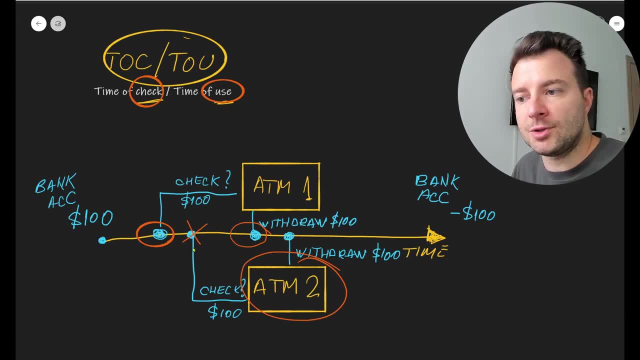 going to access it and be presented with a false representation of the state of the resource, And what I mean by somebody else is probably going to be another thread, another process, maybe another user trying to access the same resource, Another situation where a race, condition, exploit can. 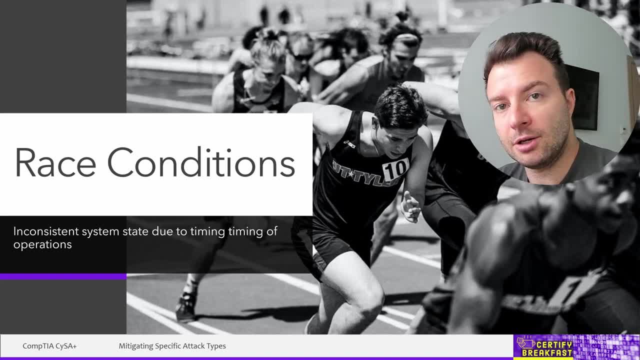 happen is if an application uses a cache file, ideally located on the user's device, and uses that cache to store a temporary file or a temporary value for future use. Now, if the user or an attacker manages to change that value between the time that the value is stored in the cache and the 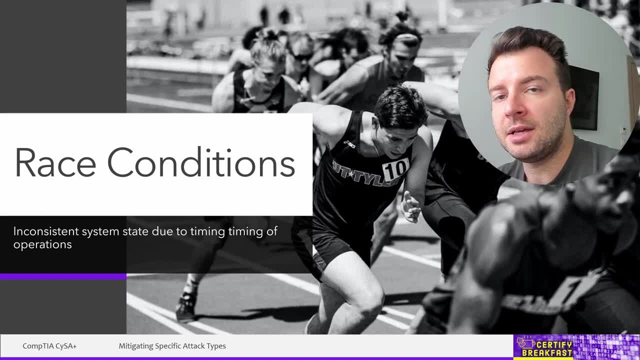 time the value is used from the cache. this is exactly the type of race condition exploit that we're talking about. So the solution is to try to change the value of the cache and the time the value is stored in the cache. You can also try to define atomic operations in your code operations. 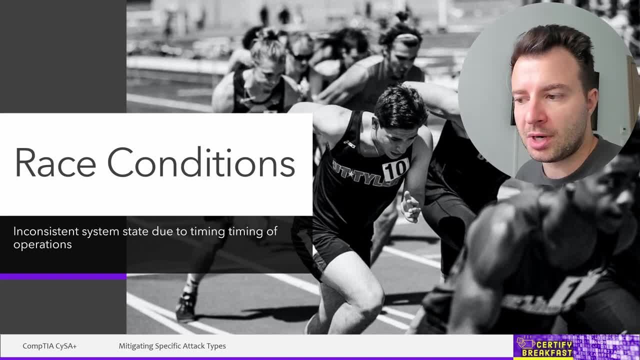 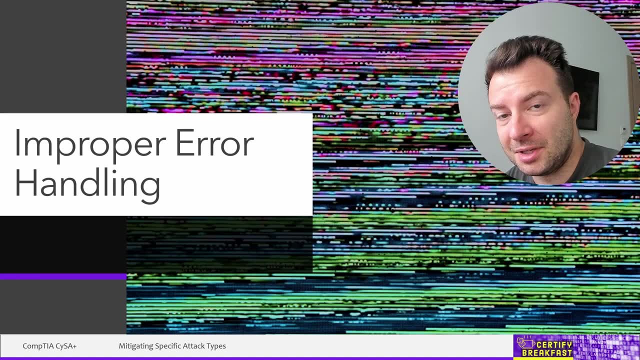 that either execute entirely or not at all. In other words, don't program sequential independent operations when they could have been done together. Another one on the list of coding vulnerabilities is improper error handling. Now, before we talk about what's proper and what's improper about error, 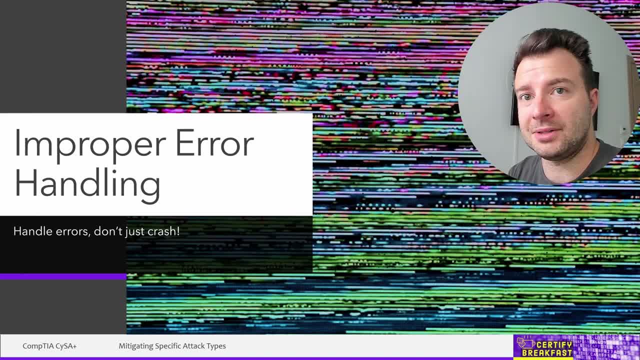 handling. please make sure that you do handle errors in your applications. Don't just let the application crash into an unknown error curve, For example. you can handle a certain error curve. it gives you an error but it's not a good err. For example, let's say your code is taking a wrong oder. 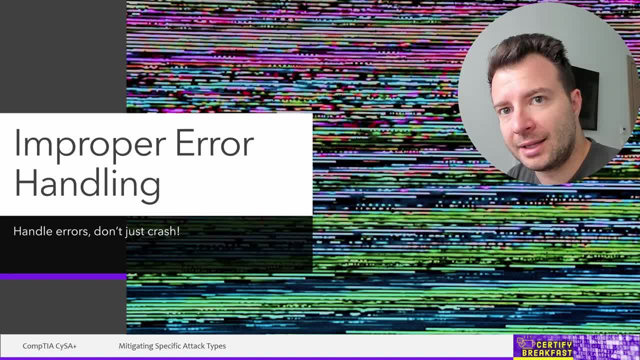 and you just change the value by changing the value of the error curve, Then it gives you an error error curve in unknown state. make sure you catch those errors beforehand and you have some piece of code that handles that specific situation. Catching errors is called exception handling and it is done using 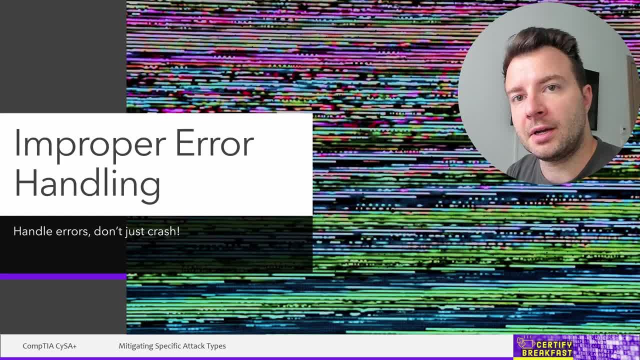 special code that is executed when a specific error situation or condition is detected. That's the code where you decide what you're about to do next instead of just crashing the application, And since, of course, you cannot just prepare for any kind of possible crash scenario that might. 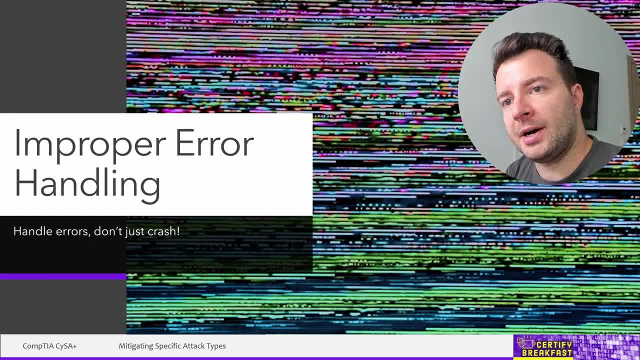 cause your application harm. there's also a way to define in most programming languages sort of a catch-all exception. So if it doesn't match any of the known or expected conditions for errors, we also have a generic code that's going to handle any other type of condition that. 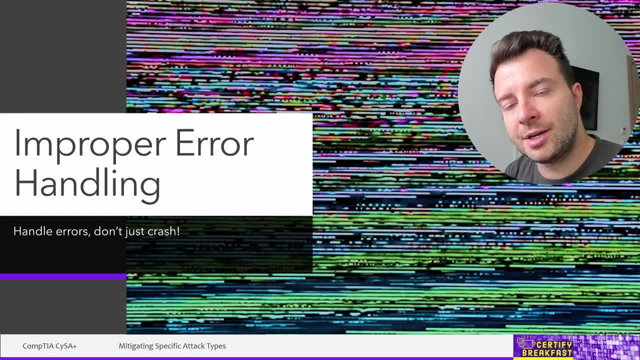 can lead to an application crash. So bottom line here: try to fail gracefully right, Don't just let the application crash. handle that situation using your own code. The point is that crashing an application is always a good thing, but it's also a good thing if you don't have a good. 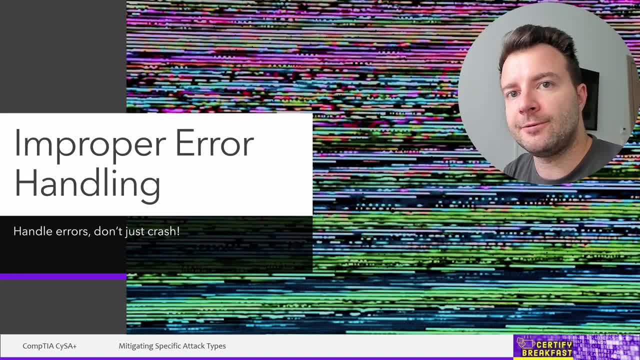 and can leave your application in a very insecure state, which is very bad for cyber security. Also part of the exception handling code: make sure you deallocate memory when the exception occurs. Don't leave important data in memory when you don't know exactly in which state your 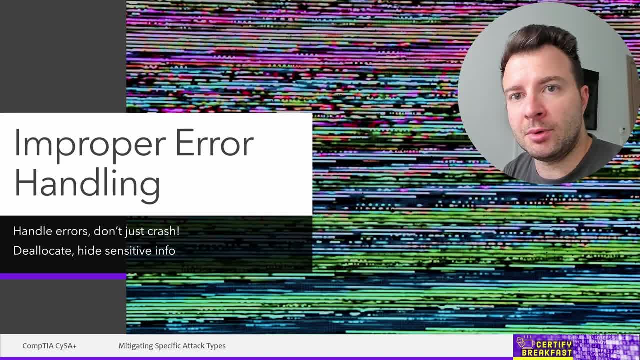 application might end up. Also, don't provide just to anyone, to any user, things like debug information. Don't fall back to default configurations or to default pages. Don't provide static data to any user. Don't provide static data to any user. Don't provide static. 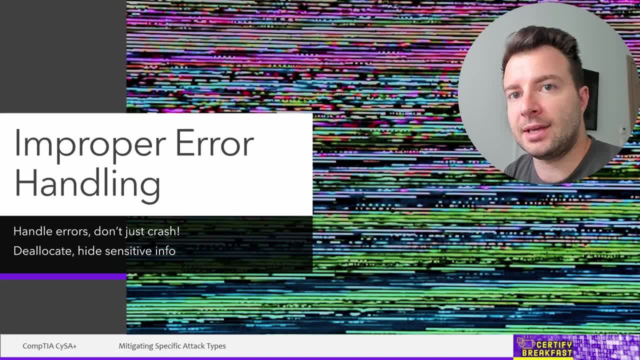 traces or the full SQL statement that caused the error. Don't provide more information to a potential attacker than they should be aware of. It might be irrelevant information for a normal user, but it might be a goldmine for an attacker who just found out more about the backend of your 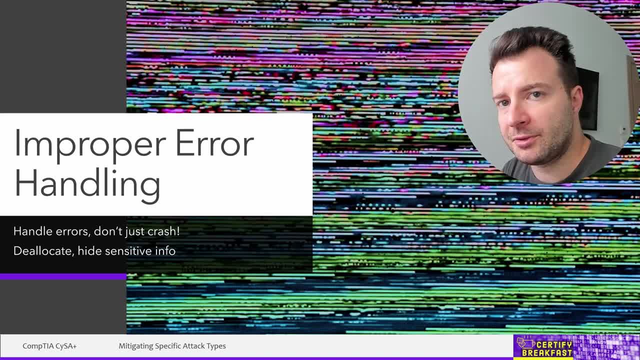 application- And I know I've said this before a number of times- don't provide detailed authentication error details. So if it's just the username, that's bad. Don't tell this to the user. If it's just a user, don't tell this to the user. Just tell him authentication failed, That's it. Don't provide more. 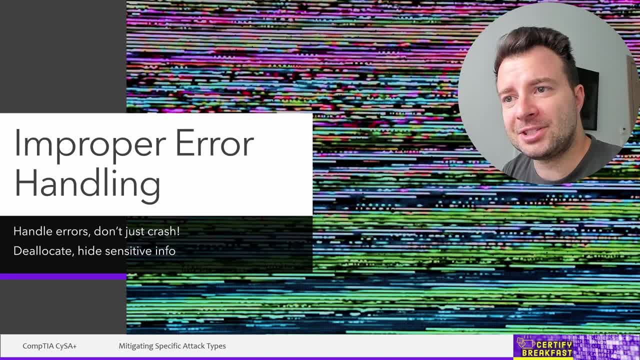 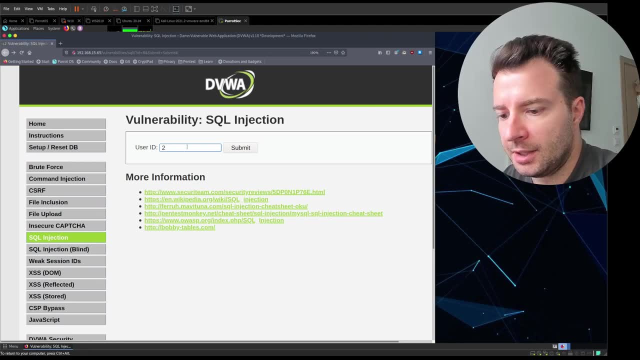 information, The more information you provide. you're basically telling an attacker: you did not attack me, right? This is what I expected. You don't want to do this. Now, here's an example here of badly managed errors. So, for example, in this field right here, if I add something like user ID 2,, 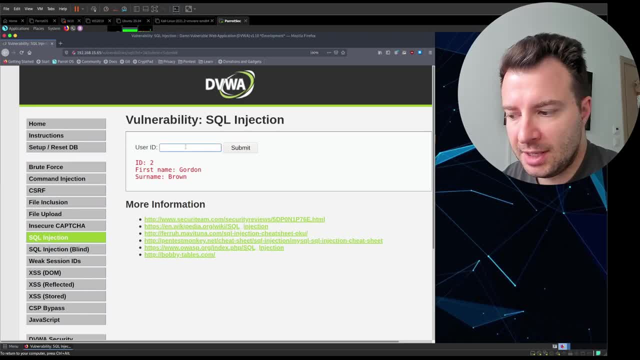 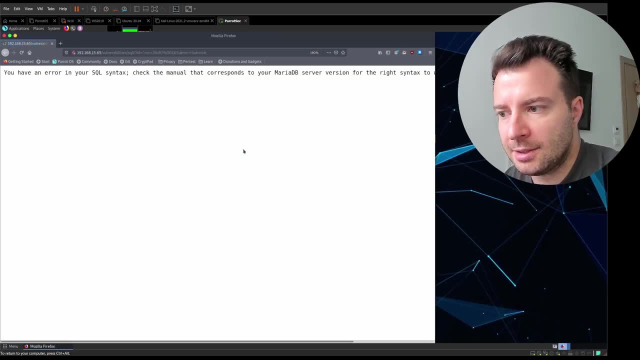 right and press enter. well, I'm going to get some information about that user ID. But if I try to do a slightly easy SQL injection attempt in here and I click submit, the end result is that I'm going to be shown. 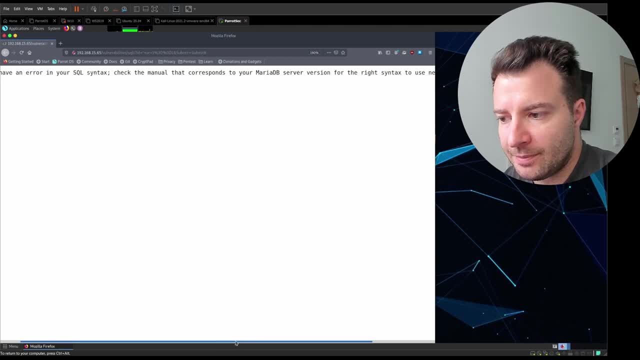 the exact error generated by the database engine in the site. So, at the very least, I just found out that the backend is actually a MariaDB server. There you have it. We did not know this a couple of seconds ago. Why would you tell this to any average user that would access your website? 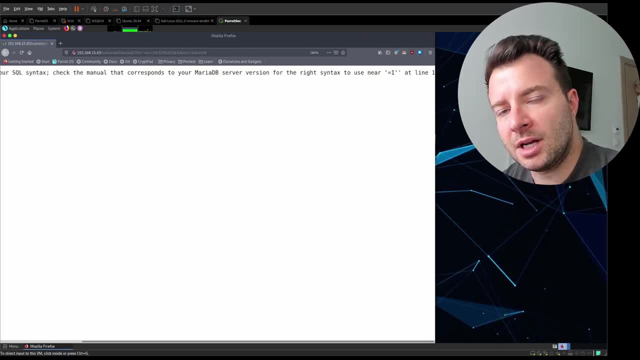 This is not relevant information for them. I'm sure you can remember a lot of websites where you accidentally mistyped some information and you ended up seeing some part of the SQL statement that generated that error. That's also part of badly managed input validation. 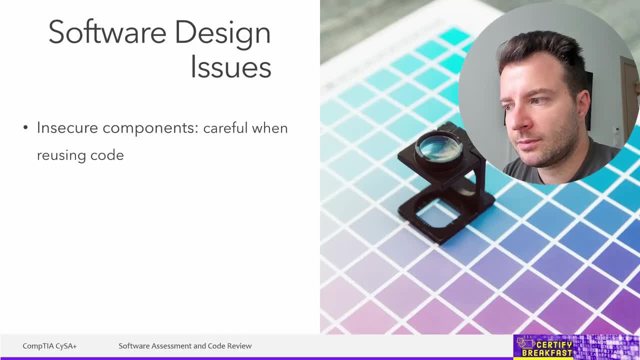 and also badly managed error handling as well. Okay, moving on to other software design issues that can lead to vulnerabilities, One of them being using insecure components. Well, developers don't like to reinvent the wheel. So, on each new software project, on each new feature, well we're. 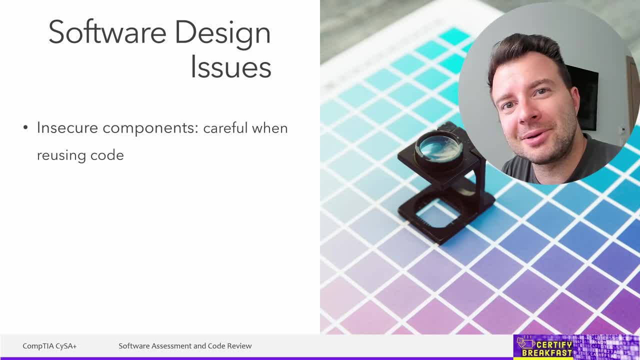 going to look for somebody else who has invented the wheel before us. so we're going to reuse some libraries, some code that wasn't perhaps thoroughly analyzed for vulnerabilities. So careful when reusing code, And this also applies to third party libraries and their vulnerabilities as well. 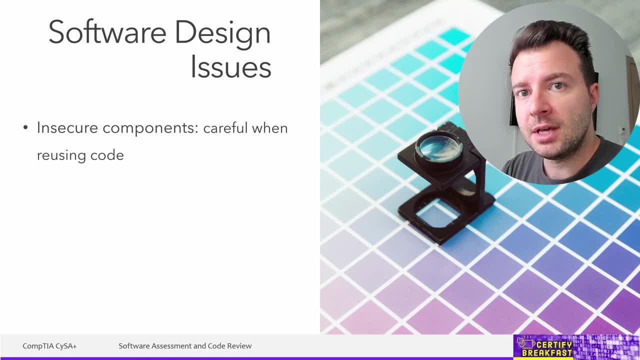 SDKs, or software development kits that are sometimes used by developers, most often include some sample codes, some sample applications that are used as the code skeletons for the future application. 001, 001, 002, 003, 004, 005, 007, 006, 007. 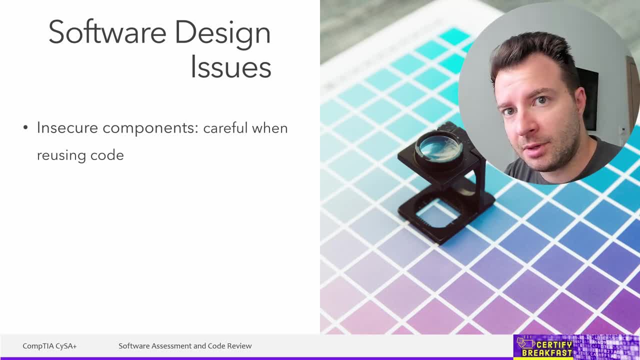 007, 008, 0010, 0011, 0012. samples were not designed with security in mind, so any problems, any vulnerabilities that were in the sample code from the very beginning might end up in the file code at the end of the project. and even if you're, you're thinking well, i'm not a programmer, i don't need to worry about this. 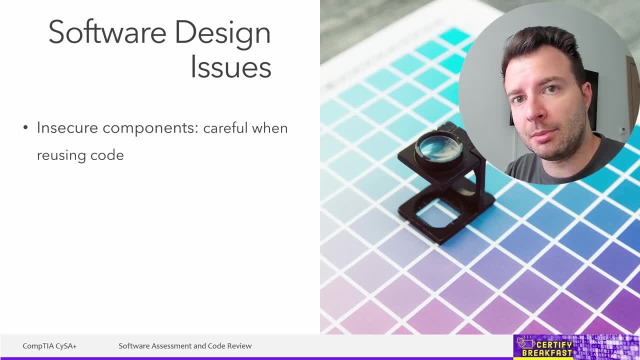 well, even if you're just managing a website, that website is probably going to be using something like joomla or wordpress and you're going to be using themes and plugins that you download from the internet. well, that's actual code that you're reusing and that might have certain vulnerabilities. 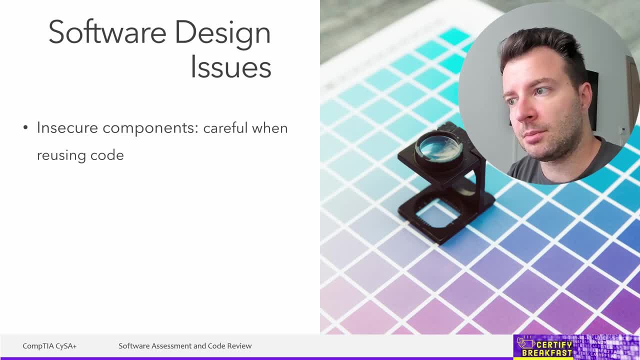 so, if you must use third-party code, think about some mitigating control, for example, like a web application firewall that can put in front of your web servers and can protect you from well-known web oriented attacks. secondly, we have insufficient logging and monitoring and a lot of security. 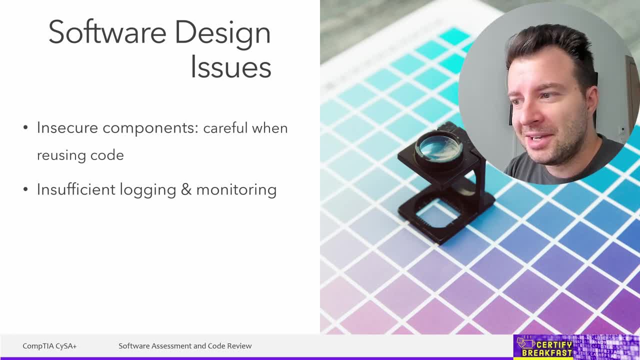 incidents are detected and eventually avoided thanks to the magic of logging and monitoring, and a lot of security incidents are detected and eventually avoided thanks to the magic of logging and recording all the events that happened when it happened, who was responsible? what was affected? so make sure you log the behavior of your applications, but be careful not to log too. 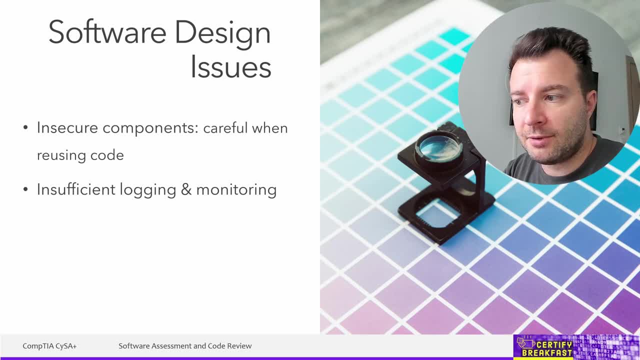 much information so that it becomes unmanageable. at the very least, design your logging mechanism to store at least information regarding, you know, successful operations, failed operations. make sure you don't expose any sensitive information in your logs. make sure you store the input validation errors in your log so that later on you can identify any attempts. 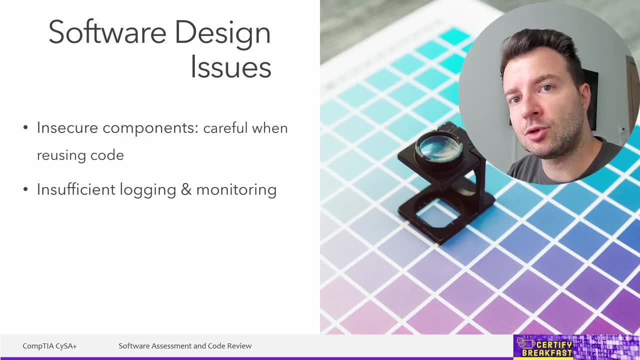 of breaching the security of your application. any abnormal events like attempts to tamper with file integrity or to access application regions that are normally inaccessible for regular users. any attempts to connect with invalid session ids that can suggest that somebody's attempting to perform some session stealing, cookie stealing session, hijacking any admin function. 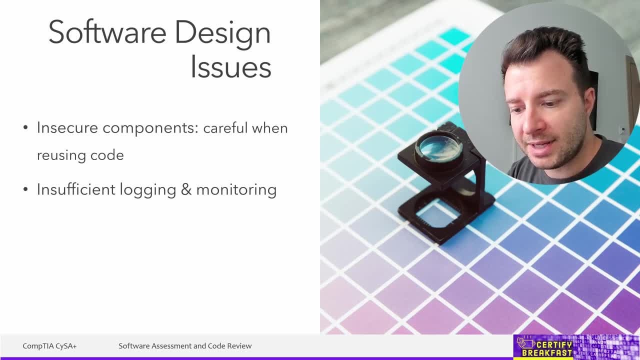 you can use to breach the security of your application. so make sure you don't expose access to the security of your account or the security of your application or your email address in your first service. that's something that you don't want to do, so don't. 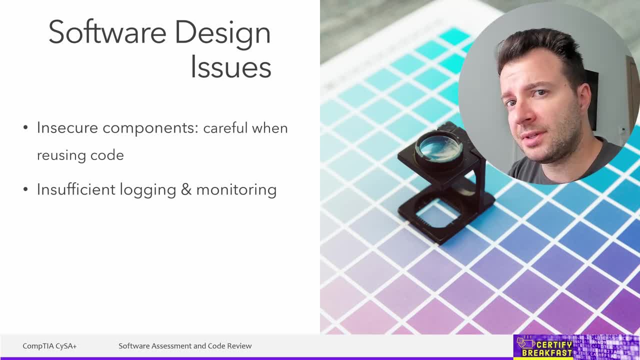 ignore usage. make sure you log everything that is recorded as being performed by an admin, just to make sure that there was an actual admin running those commands and not somebody who escalated their privileges or impersonated an admin- and i don't think i have to mention this. but restrict access to those logs. make sure that regular users cannot. 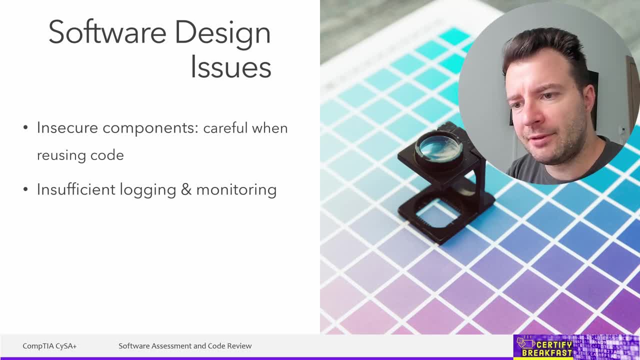 access those logs and not to mention make sure that they are not able to change or write, sound like a trivial habit. you know the type of work that nobody wants to do. But having continuous monitoring is very useful, especially when your company doesn't really have a strong. 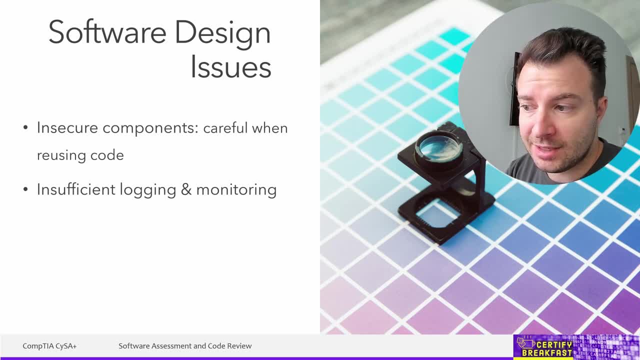 security posture. Now, the chances are that when you get compromised, you will find out after the incident has happened, And if you don't have the proper monitoring tools in place, you might not even know how it happened and what you need to do in the future to avoid finding yourself in the 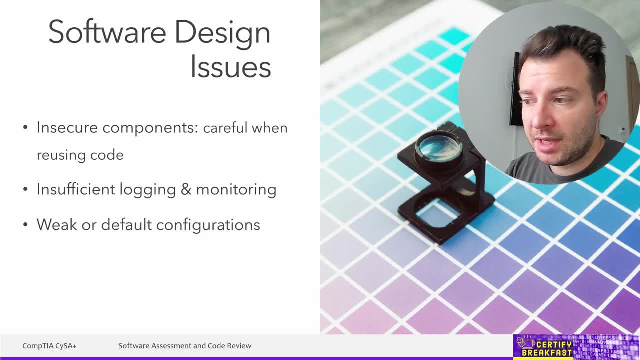 same situation to avoid being breached in the future as well. Then we have weak or default configuration, And the main idea here is that, regardless of how secure the code of an application is, if an admin or a privileged user decides accidentally to expose some sensitive information. 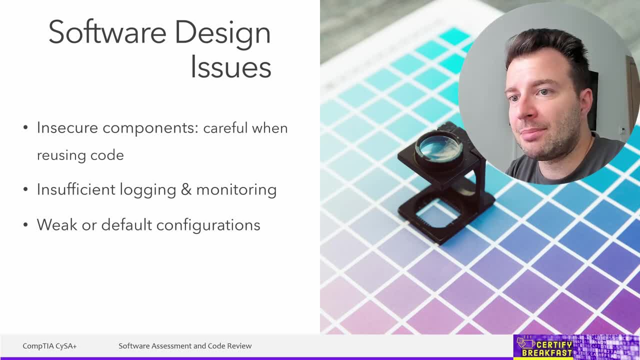 well, that's a vulnerability that was introduced from the application's configuration. So sometimes it's a vulnerability that was introduced from the application's configuration. So sometimes it's a vulnerability that was introduced from the application's configuration So somebody misconfigured the permissions in that application and accidentally 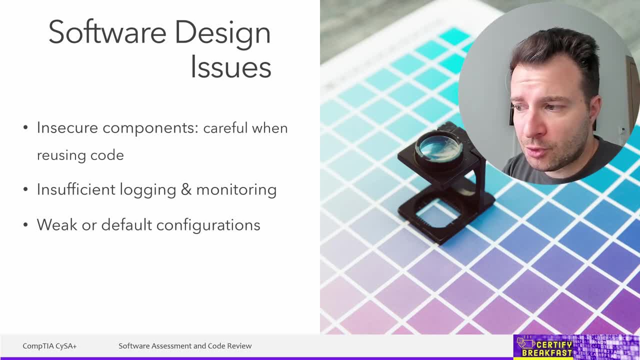 exposed something that shouldn't have been visible. Very important, don't forget about default configurations, like default configs and Wi-Fi devices and IoT devices and networking devices and I don't know your home wireless router, for example. They all have default accounts with default configurations which are well known, And there are automated tools out. 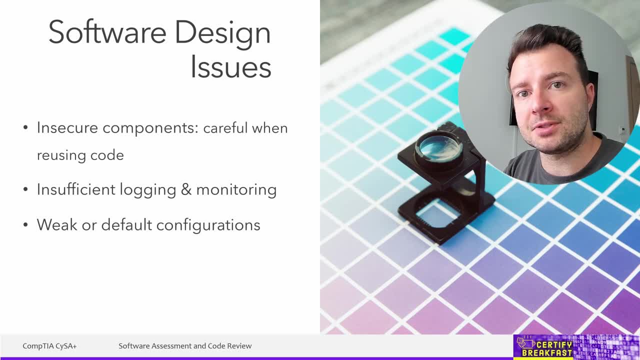 there that search for these exposed admin interfaces, exposed to the internet, and they just brute force try to connect using those default credentials And more often than not they succeed because people forget about those. So make sure you change your default configuration and your. 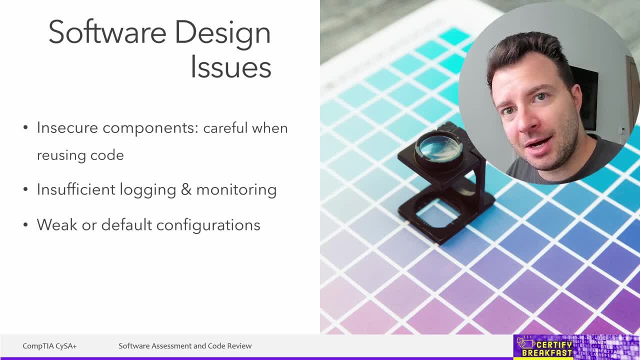 default accounts And even renaming the admin accounts is a well-known practice for just obfuscating some sensitive information, You know. try to make the attacker's life a bit harder. If every admin user all over the world would be called admin, then the attacker's job would be only to 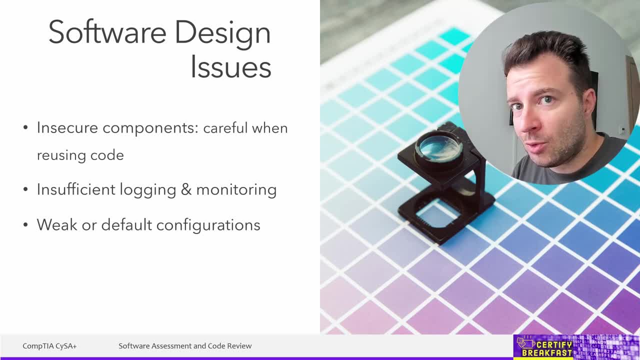 crack the password, But what if the attacker doesn't even know what is the name of the admin account? Why not use this? Finally, broken authentication. This one refers to an application that performs authentication and authorization for the user accounts that it has, but it does them badly, And this can be due to a number of 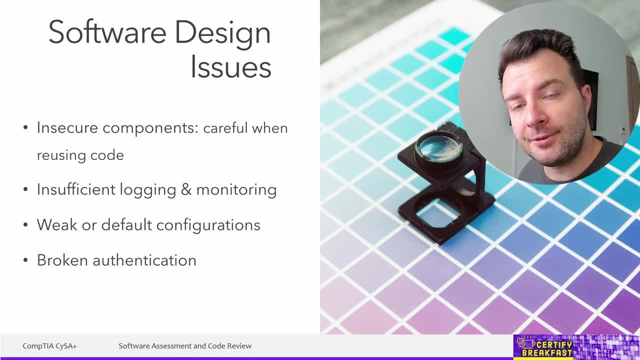 faults Like, for example, the application can accept very weak passwords, You allow your users to use very weak passwords, Or it has a very weak password reset mechanism. A badly implemented password reset would be, for example, to ask the user to provide the email address where the new reset link or 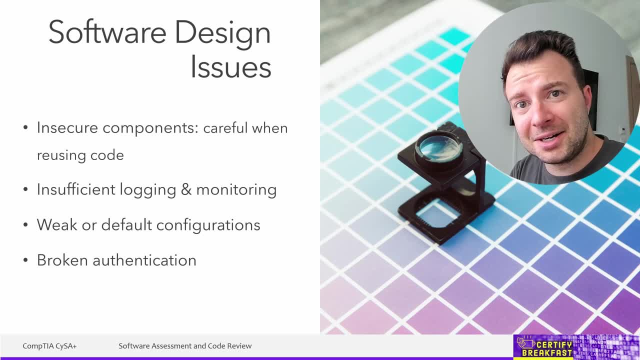 even the new password is to be sent. Now, of course, an attacker would easily be able to reset anybody's password using a mechanism like this, Or even a system that resets all passwords to the same default one. Don't laugh, you can find this in real life and it. 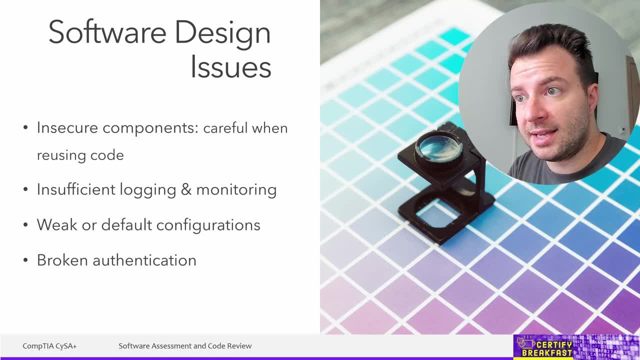 happens. Also, it might happen that the application can expose some sensitive session information. Like you know, if you have a unique session IDs, credentials or authentication tokens, Either because they're not encrypted or they are hard-coded in the application or exposed somewhere, like in the URL of the password reset link. Another situation is when the application stores all these. 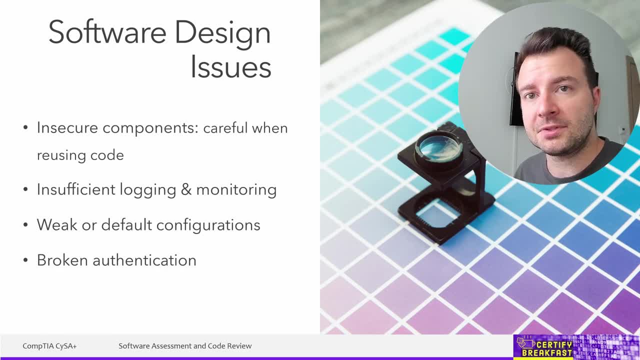 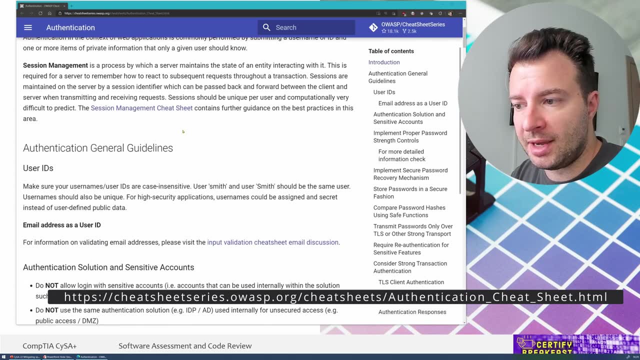 credentials in clear text which exposes them all if the system is accidentally compromised. Now for a full list of best practices. have a look over this authentication cheat sheet hosted by OWASP. It's going to provide you with a lot of guidance and cover.